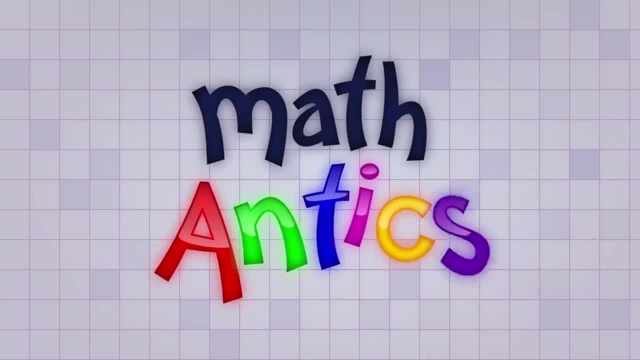 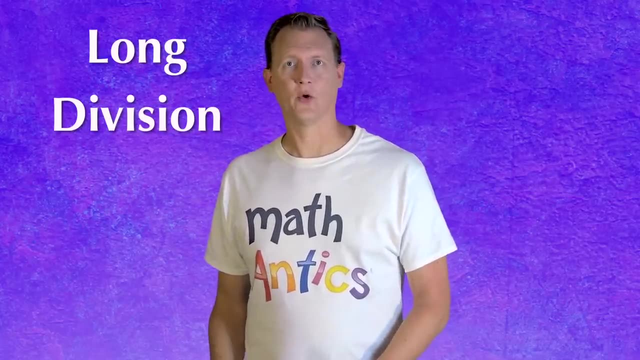 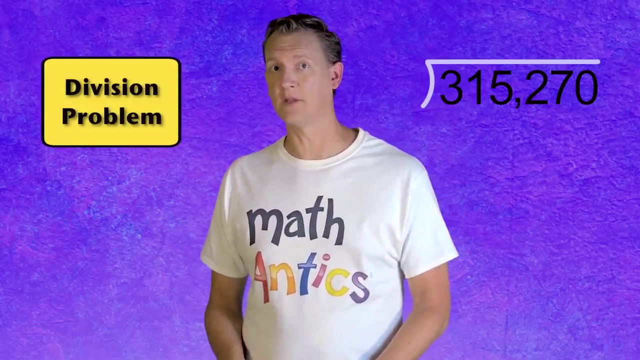 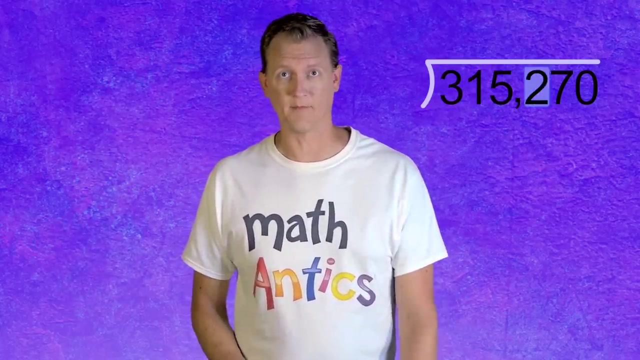 Hi, welcome to Math Antics. In our video called Long Division, we learned how to do division problems that had long, multi-digit dividends. The key was to break up a big division problem into a series of smaller and easier division steps, And that involved trying to divide the dividend one digit at a time, digit by digit. 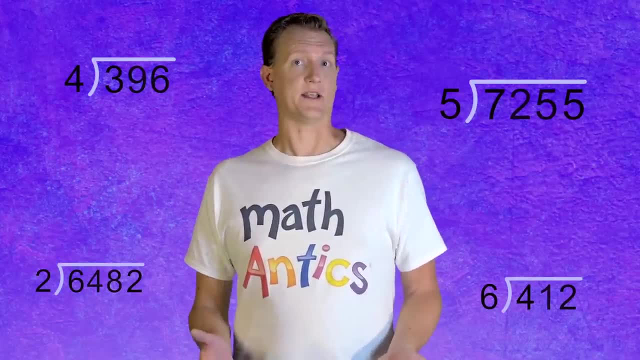 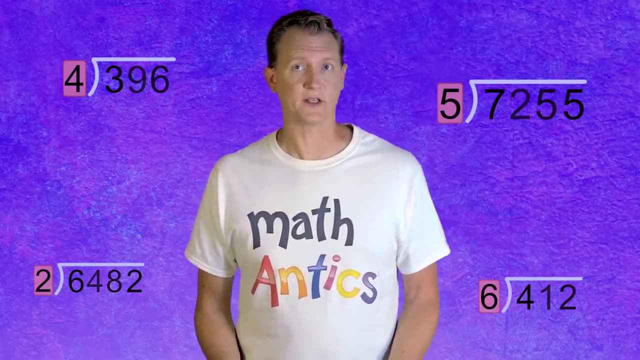 And in the examples we saw, going digit by digit was pretty easy because we only had one-digit divisors. But what if you need to use that division method for problems that have bigger divisors, like if you're dividing by a two or three-digit number? 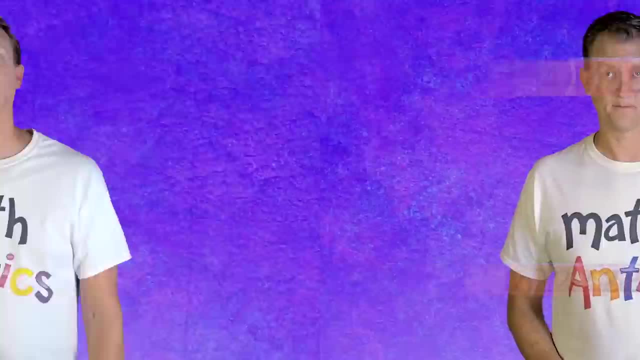 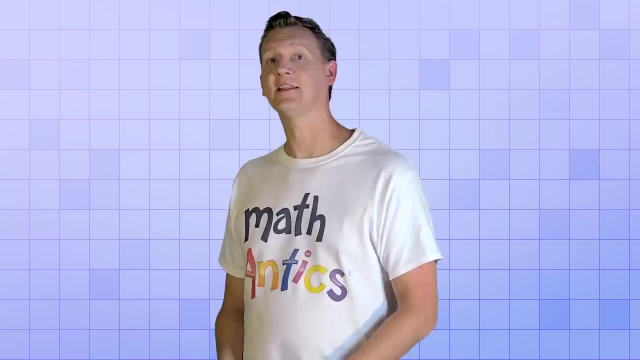 In this lesson we're going to learn how you handle problems like that. The good news is that you kind of already know what to do. you just may not realize it yet. To see what I mean, have a look at these two division problems. 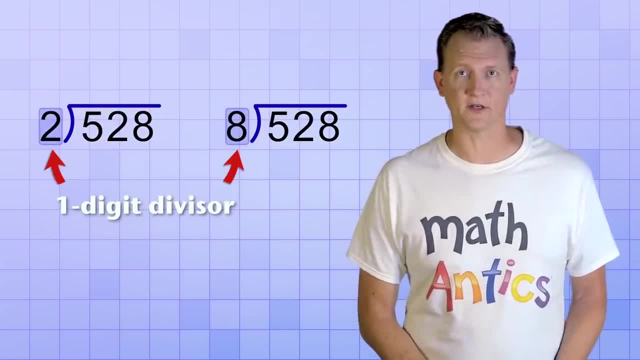 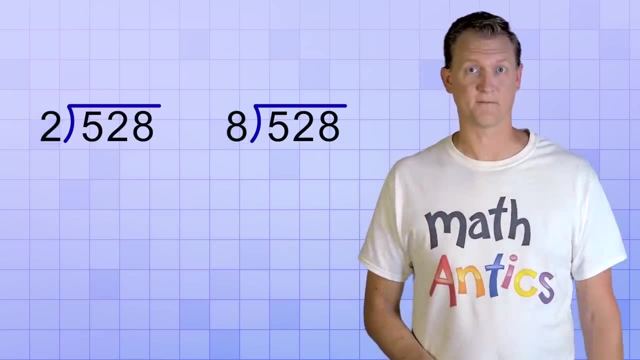 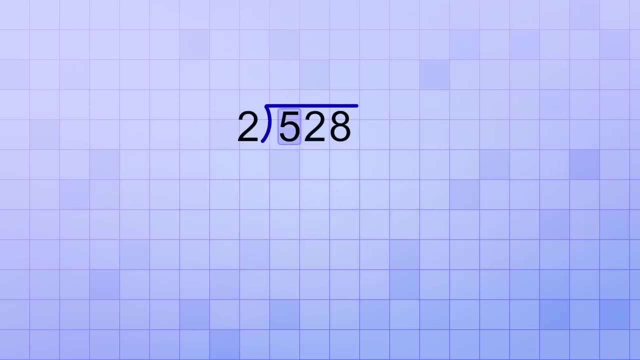 They both have the same dividend and both have a one-digit divisor, But these divisors are different numbers and, as you'll see, that's going to affect our digit by digit division process. To solve this first problem, we start by asking: how many twos does it take to make five, or almost five? 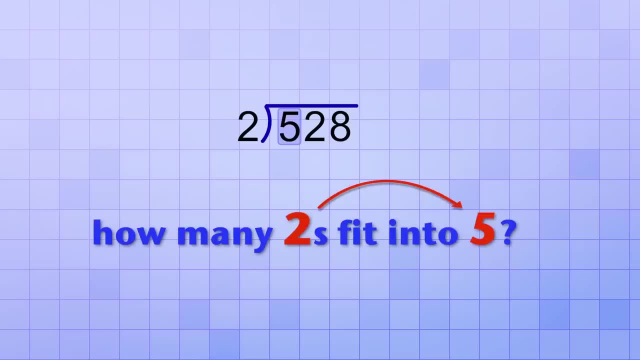 Or you can think of it as how many twos will fit into five, And it's easy to see that the answer is two. So we put a two as the first digit of our answer. Then we multiply two times two, which is four, and we subtract that four from the five. 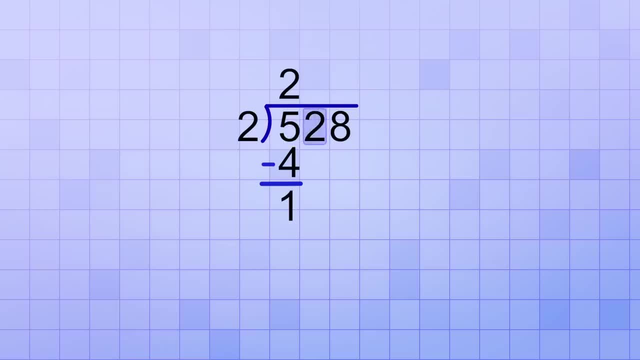 which leaves us a remainder of one. Now we move to our next digit and we need to bring down a copy of it to combine with the remainder from the first digit. Then we ask how many twos will make twelve? That's easy six. 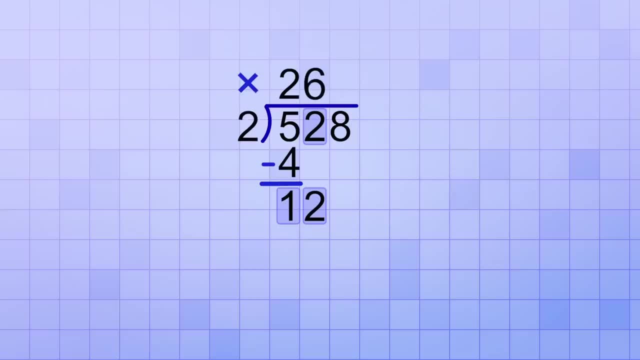 So we put six as the next digit of our answer. Two times six equals twelve, and twelve minus twelve leaves no remainder. And finally, for our last digit, even though there is no remainder, we can bring a copy down and ask how many twos will make eight. 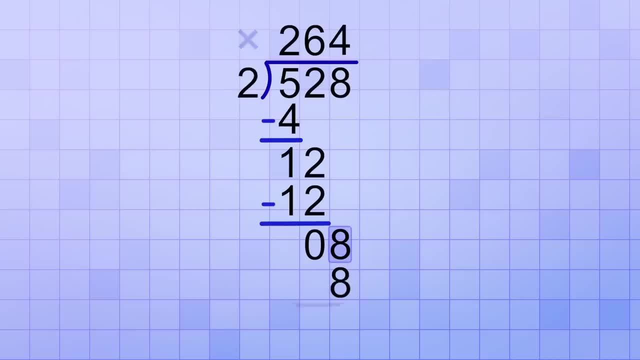 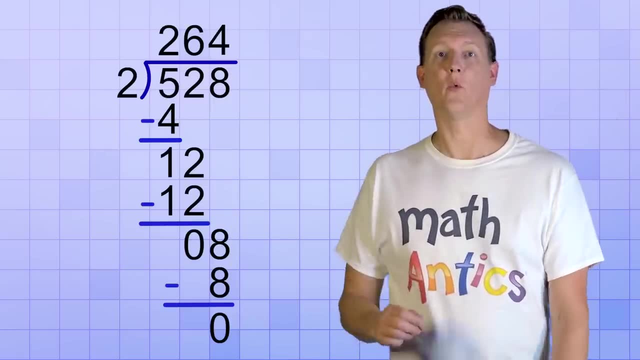 The answer is exactly four. Four times two equals eight, which again leaves no remainder. There we went digit by digit and broke our problem up into three division steps, one for each digit, And we got our answer two hundred and sixty-four. 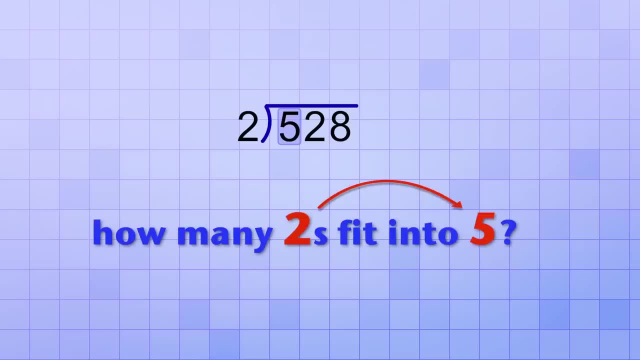 Or you can think of it as how many twos will fit into five, And it's easy to see that the answer is two. So we put a two as the first digit of our answer. Then we multiply two times two, which is four, and we subtract that four from the five. 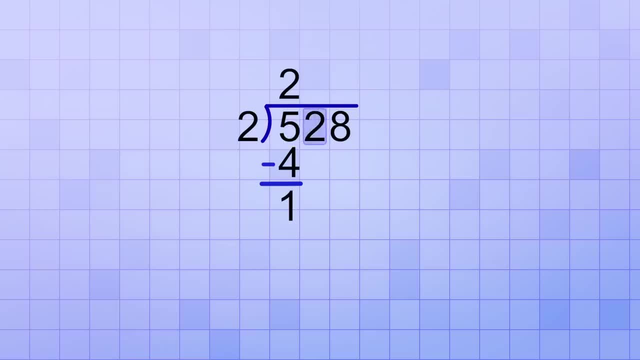 which leaves us a remainder of one. Now we move to our next digit and we need to bring down a copy of it to combine with the remainder from the first digit. Then we ask how many twos will make twelve? That's easy six. 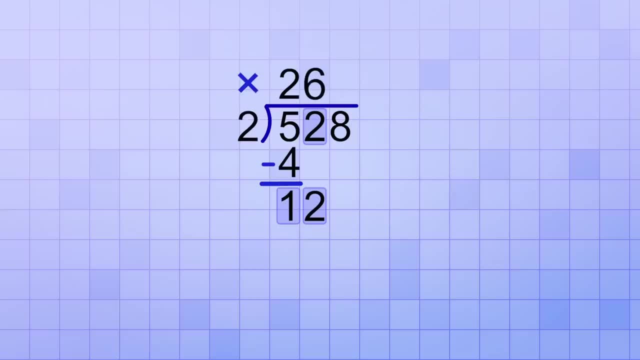 So we put six as the next digit of our answer. Two times six equals twelve, and twelve minus twelve leaves no remainder. And finally, for our last digit, even though there is no remainder, we can bring a copy down and ask how many twos will make eight. 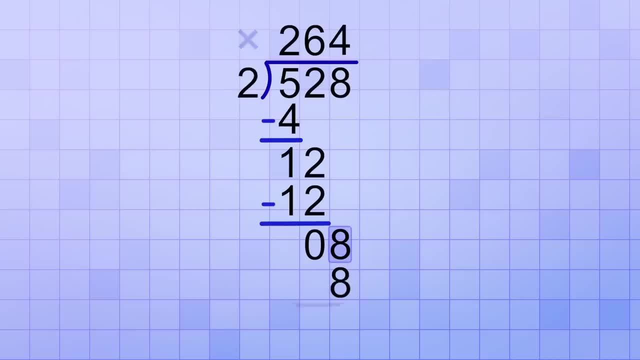 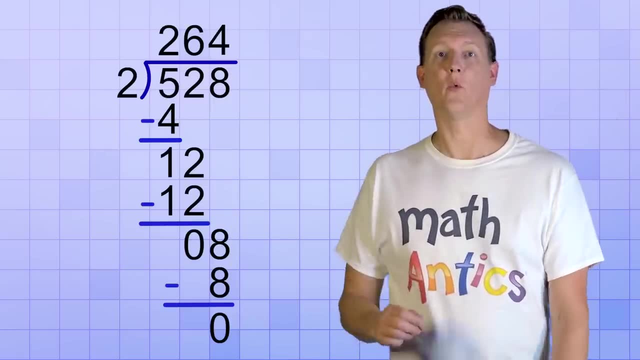 The answer is exactly four. Four times two equals eight, which again leaves no remainder. There we went digit by digit and broke our problem up into three division steps, one for each digit, And we got our answer two hundred and sixty-four. 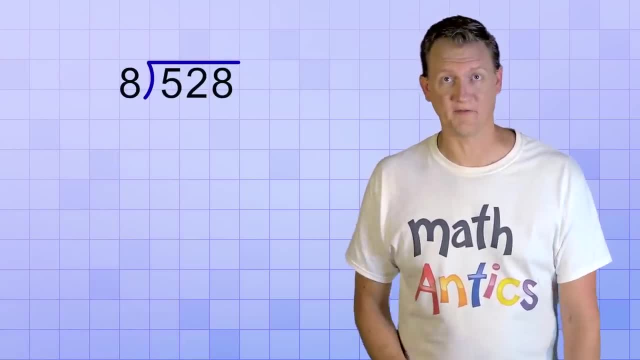 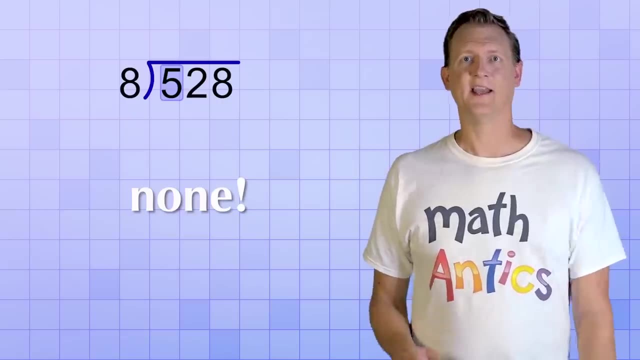 Now let's solve the next example, And right at the start you'll see, we have a bit of a problem. When we ask how many eights does it take to make five or almost five? the answer is none, And that's because the first digit, taken by itself, is less than the divisor. 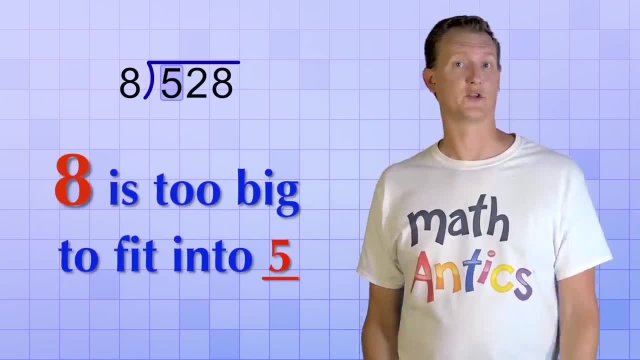 And that's because the first digit taken by itself is less than the divisor, And that's because the first digit taken by itself is less than the divisor. Eight is too big to divide into five, so what do we do? 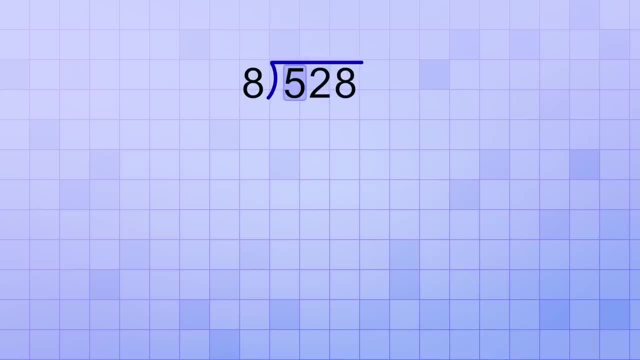 Well, instead of just trying to divide the first digit all by itself, let's group the first two digits together. If we group the five and the two together, then our first step will be to ask how many eights will make fifty-two. 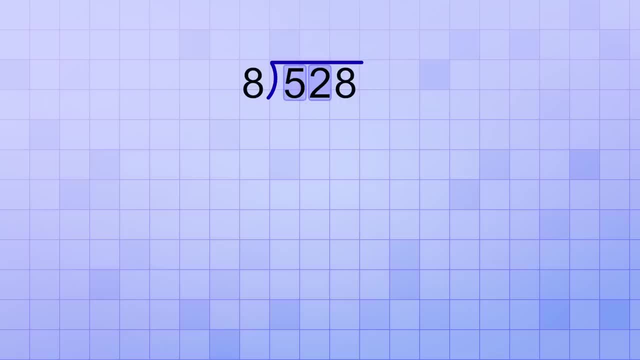 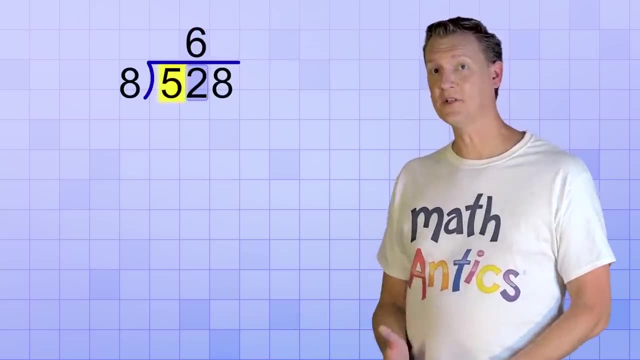 That's better. Eight will divide into fifty-two, about six times, so we'll put a six in our answer line right above the two. Why does it go there? Because we had to skip the first digit and group it with the two. 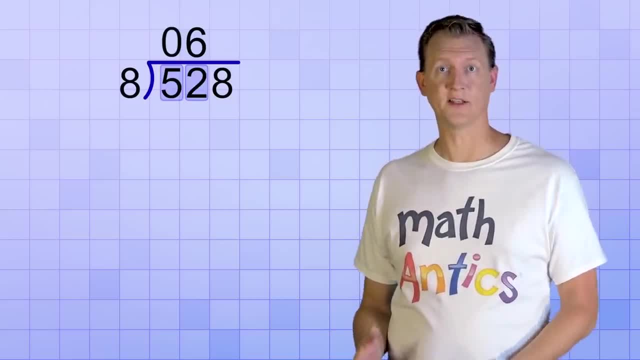 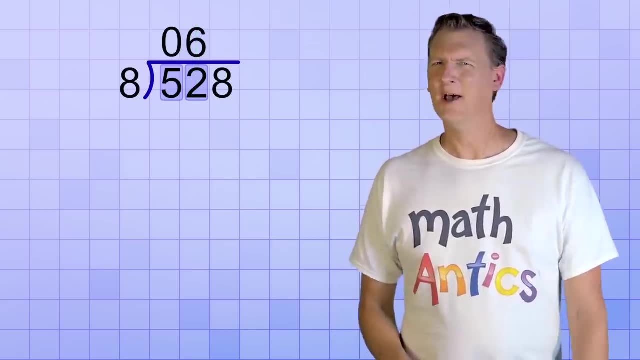 If we wanted to, we could have put a zero above that first digit, since the eight wouldn't divide into it any times. And if that helps you keep track of which answer digit you're on, then that's a good idea, But it's not required. 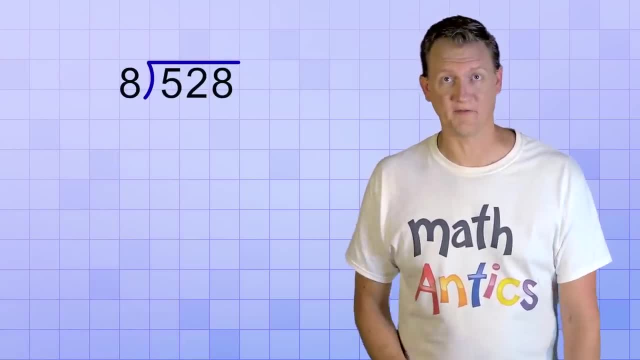 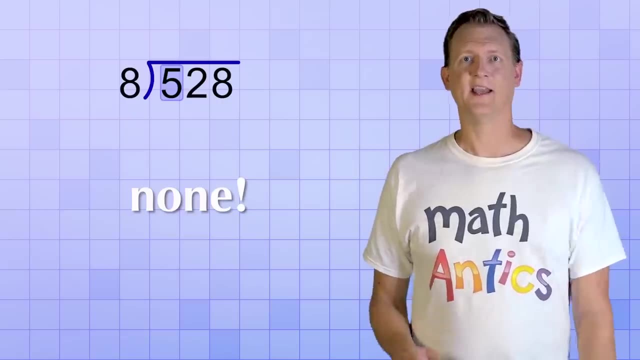 Now let's solve the next example, And right at the start you'll see, we have a bit of a problem. When we ask how many eights does it take to make five or almost five? the answer is none, And that's because the first digit, taken by itself, is less than the divisor. 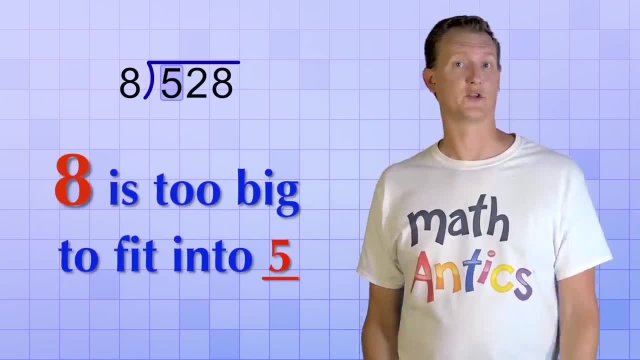 And that's because the first digit taken by itself is less than the divisor, And that's because the first digit taken by itself is less than the divisor. Eight is too big to divide into five, so what do we do? 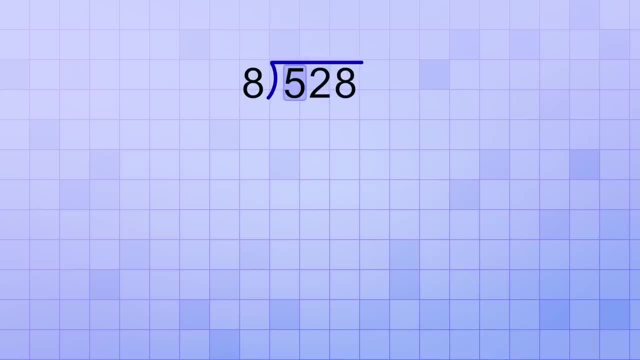 Well, instead of just trying to divide the first digit all by itself, let's group the first two digits together. If we group the five and the two together, then our first step will be to ask how many eights will make fifty-two. 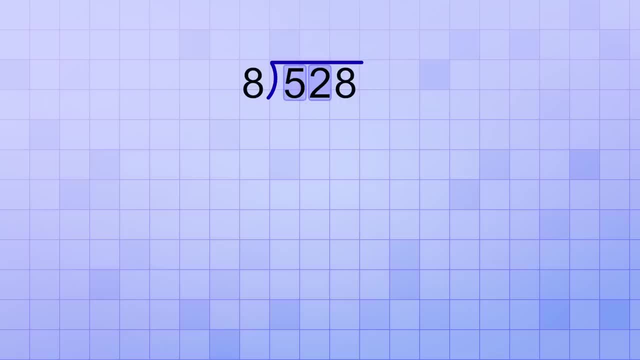 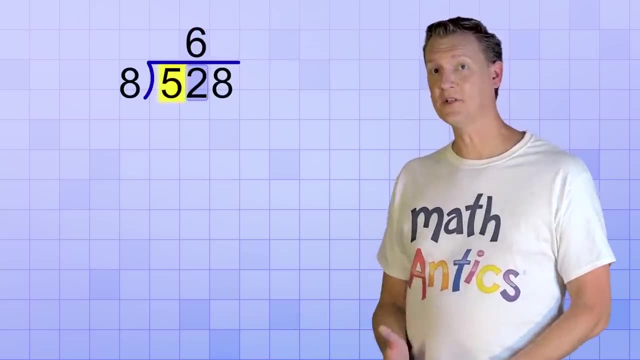 That's better. Eight will divide into fifty-two, about six times, so we'll put a six in our answer line right above the two. Why does it go there? Because we had to skip the first digit and group it with the two. 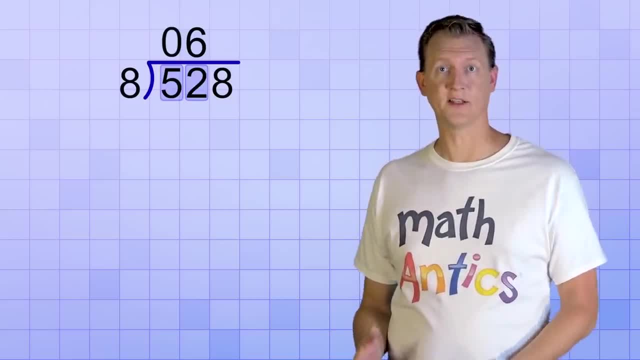 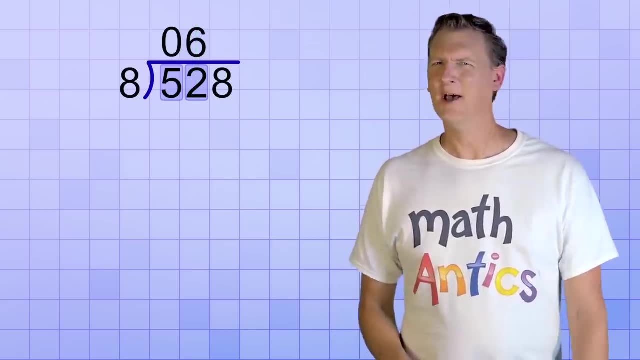 If we wanted to, we could have put a zero above that first digit, since the eight wouldn't divide into it any times. And if that helps you keep track of which answer digit you're on, then that's a good idea, But it's not required. 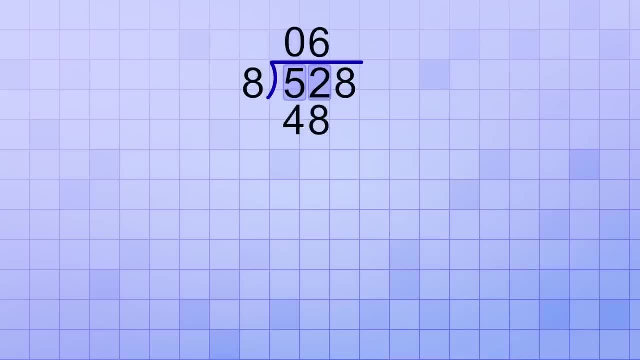 So six times eight equals forty-eight, and then fifty-two minus forty-eight gives us a remainder of four. Now we only have one digit left to divide, so we bring down a copy of it to combine with the remainder and ask how many eights will make forty-eight. 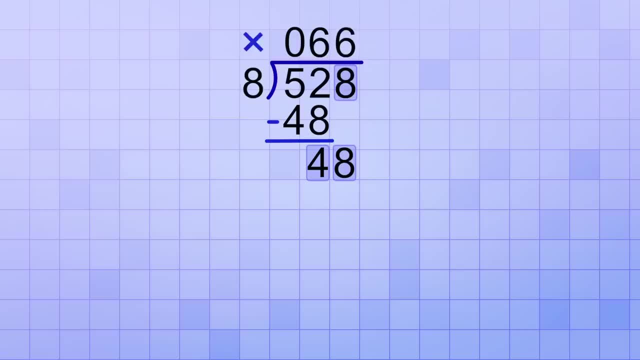 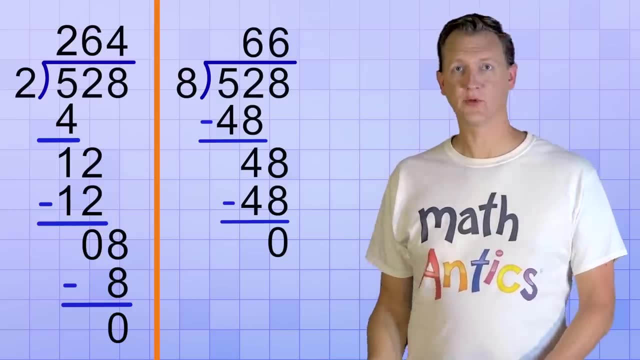 We know the answer to that is six. also, Six times eight is forty-eight, which leaves no remainder There. our answer is sixty-six. Did you notice the difference between these two problems? We wanted to go digit by digit in both problems. 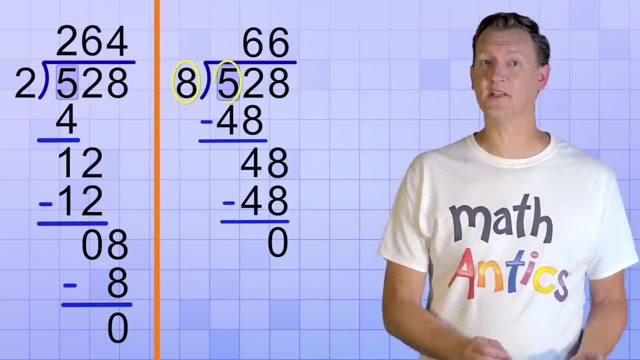 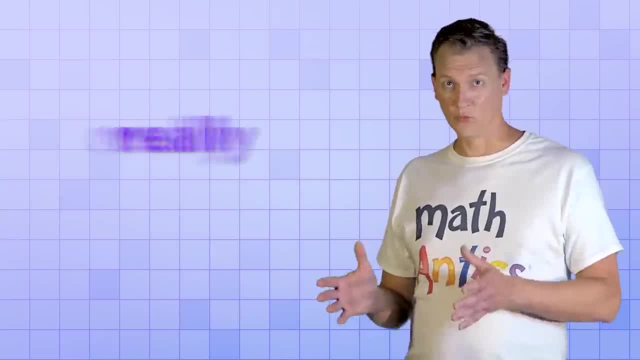 But in the second problem, the divisor was bigger than the first digit of the dividend, so we had to start out by going two digits at a time. in that case- And that helps us see something really important about this traditional long division method- You don't always have to go one digit at a time. 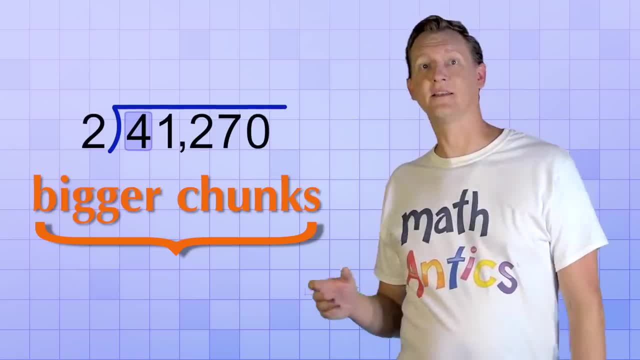 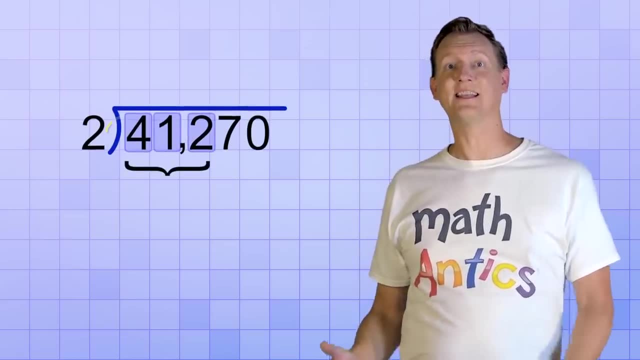 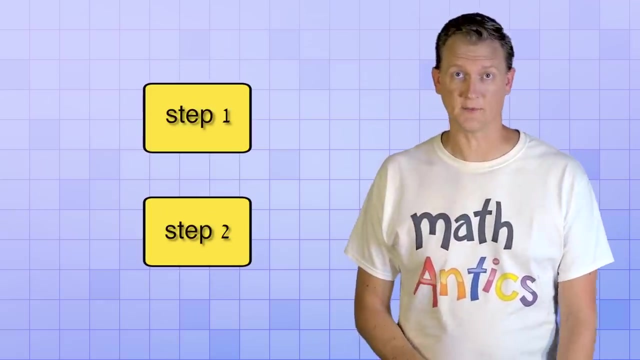 Break the dividend up into bigger chunks of digits if you want, and apply the same procedure to those bigger chunks. You could go two or three digits at a time Or even try to divide the entire dividend all in one step, And taking bigger chunks of the dividend usually results in fewer division steps. 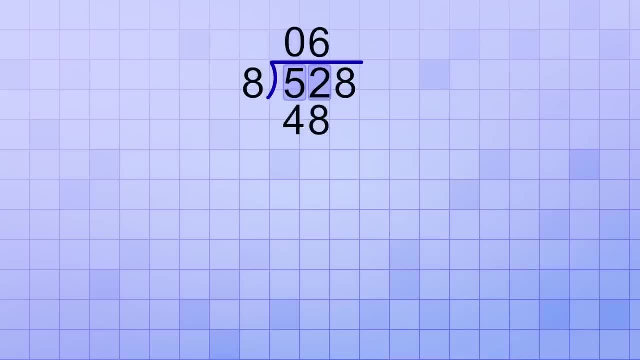 So six times eight equals forty-eight, and then fifty-two minus forty-eight gives us a remainder of four. Now we only have one digit left to divide, so we bring down a copy of it to combine with the remainder and ask how many eights will make forty-eight. 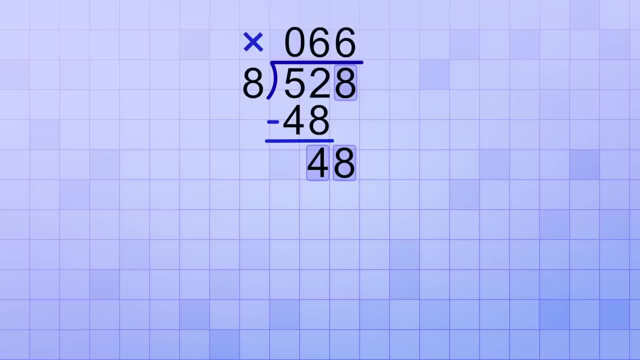 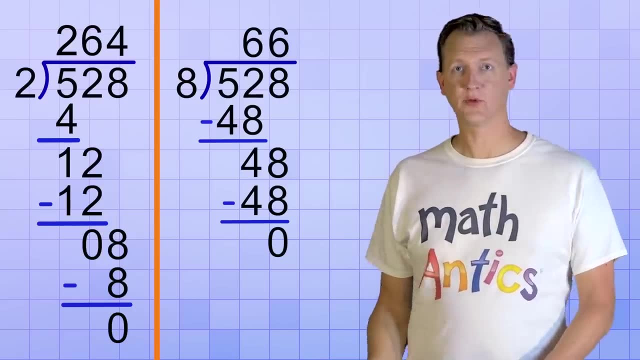 We know the answer to that is six. also, Six times eight is forty-eight, which leaves no remainder There. our answer is sixty-six. Did you notice the difference between these two problems? We wanted to go digit by digit in both problems. 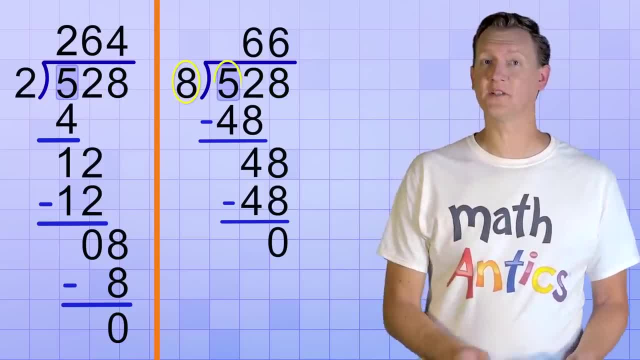 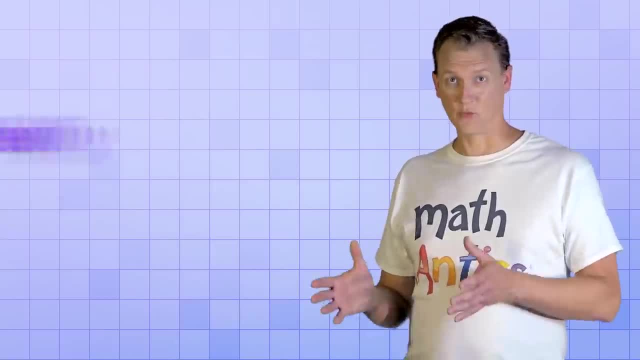 But in the second problem, the divisor was bigger than the first digit of the dividend, so we had to start out by going two digits at a time. in that case- And that helps us see something really important about this traditional long division method- You don't always have to go one digit at a time. 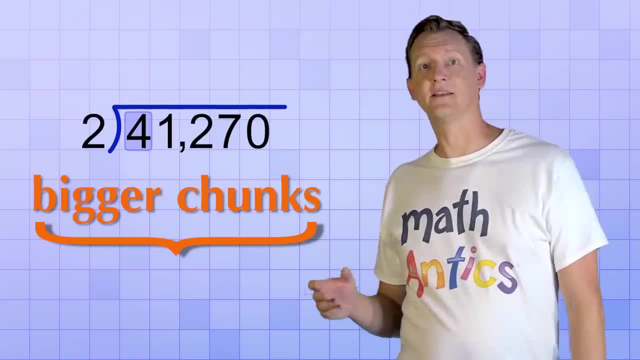 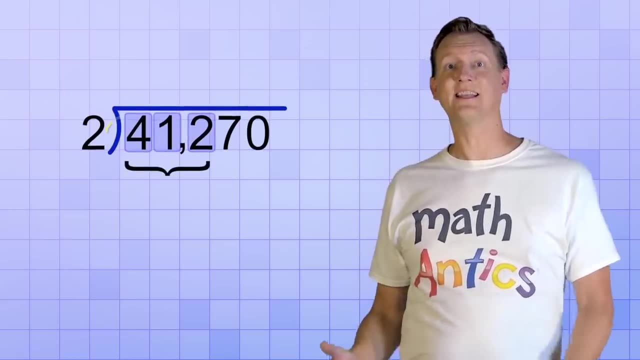 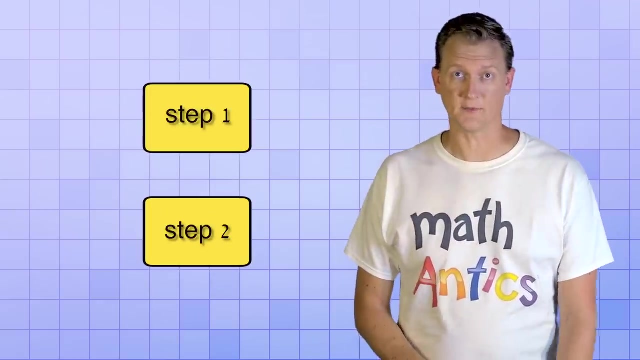 Break the dividend up into bigger chunks of digits if you want, and apply the same procedure to those bigger chunks. You could go two or three digits at a time Or even try to divide the entire dividend all in one step, And taking bigger chunks of the dividend usually results in fewer division steps. 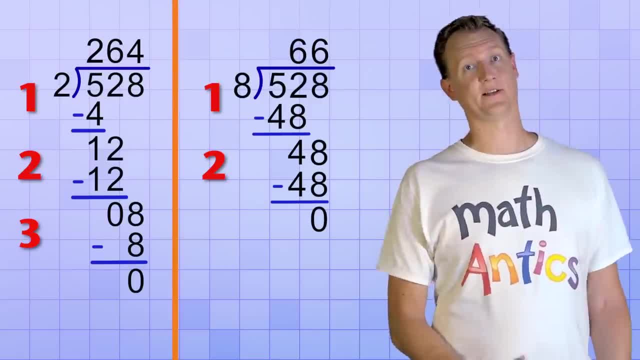 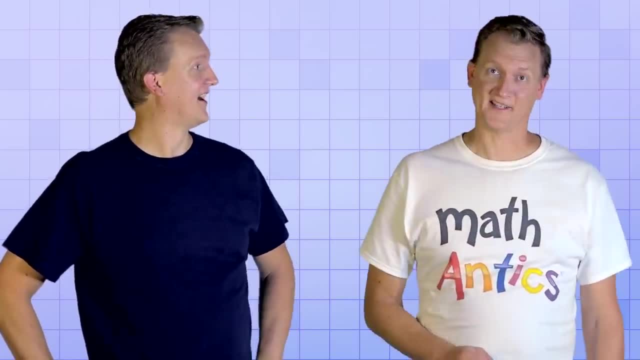 Notice that there were three steps in the first problem but only two steps in the second problem. Fewer steps- I like the sound of that. That seems like a lot less work. Ah yes, Fewer division steps does sound better, but it's really not. 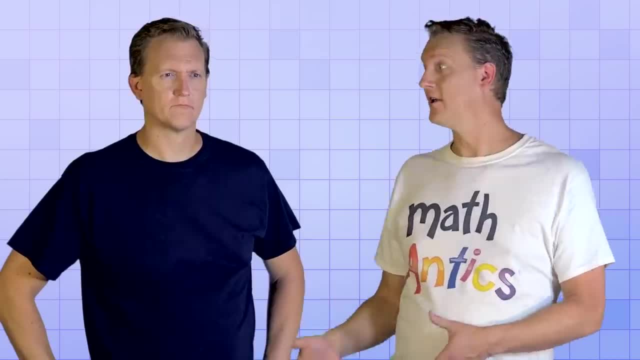 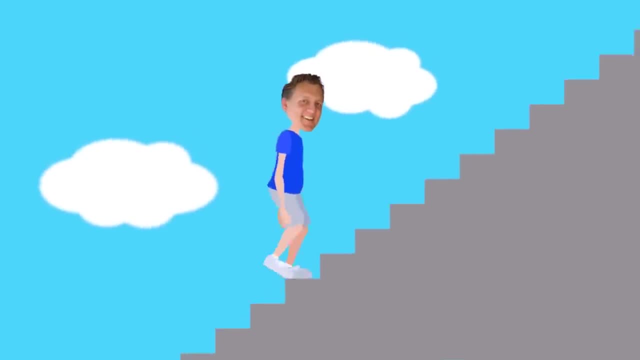 That's because the more digits you group together, the harder that division step will be. I thought it sounded too good to be true. It's kind of like climbing stairs: When you have a lot of small steps, each one is easy to climb. 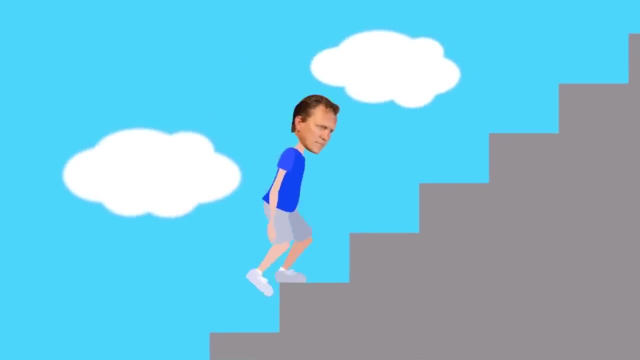 But with only a few big steps, each one can be a challenge of its own. That's why we always try to go just one digit at a time. If you only have to divide into one or two digits of the dividend, you're going to have to go one digit at a time. If you only have to divide into one or two digits of the dividend, you're going to have to go one digit at a time. If you only have to divide into one or two digits of the dividend, you're going to have to go one digit at a time. 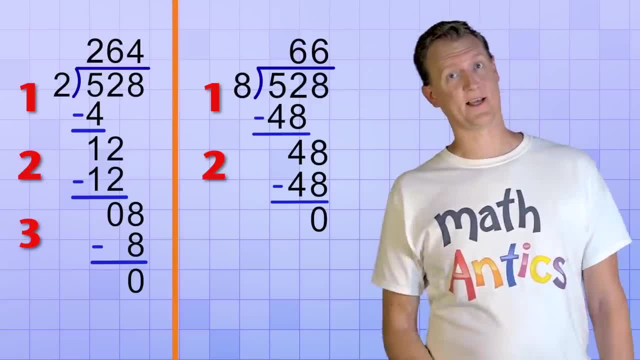 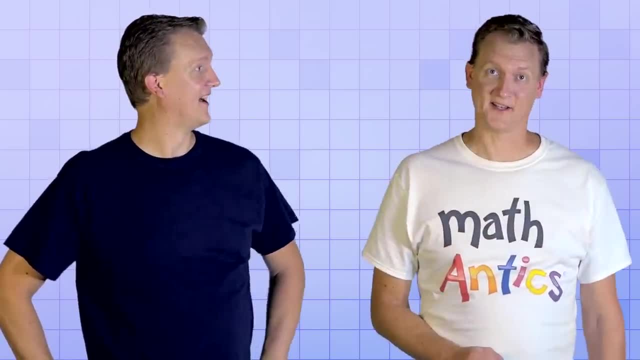 Notice that there were three steps in the first problem but only two steps in the second problem. Fewer steps- I like the sound of that. That seems like a lot less work. Ah yes, Fewer division steps does sound better, but it's really not. 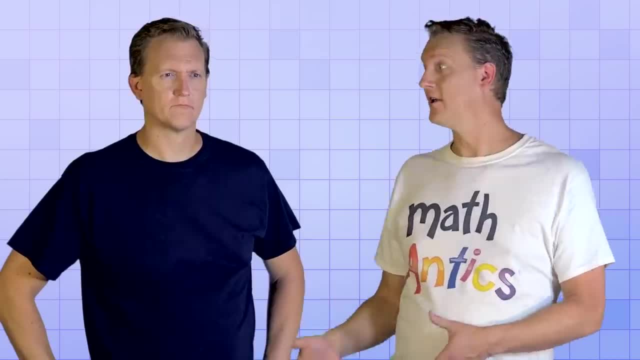 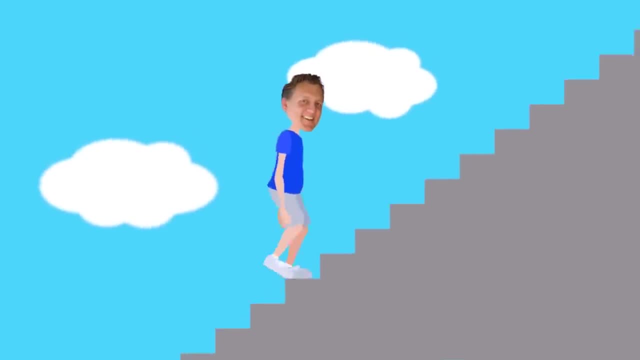 That's because the more digits you group together, the harder that division step will be. I thought it sounded too good to be true. It's kind of like climbing stairs: When you have a lot of small steps, each one is easy to climb. 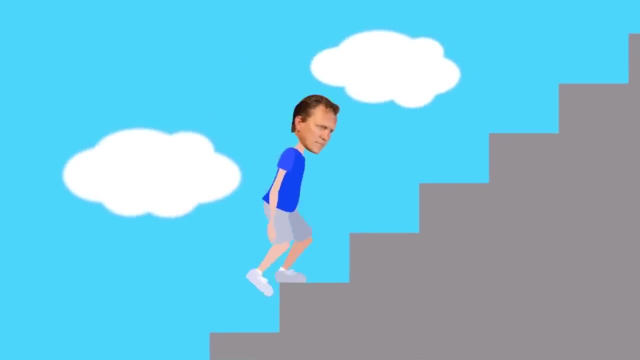 But with only a few big steps, each one can be a challenge of its own. That's why we always try to go just one digit at a time. If you only have to divide into one or two digits of the dividend, you're going to have to go one digit at a time. If you only have to divide into one or two digits of the dividend, you're going to have to go one digit at a time. If you only have to divide into one or two digits of the dividend, you're going to have to go one digit at a time. 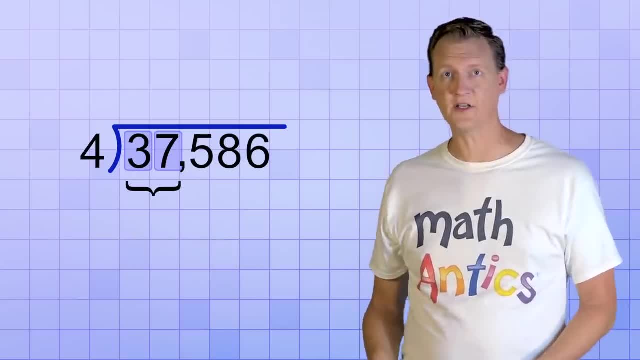 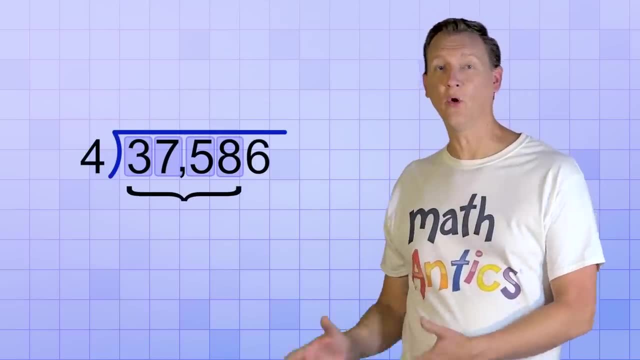 It's much easier because all of the answers to those smaller division steps can be found on the multiplication table, Which you have memorized, right, Yeah, But when we have to go three or four digits at a time, it's a lot harder to figure out the answer of each step. 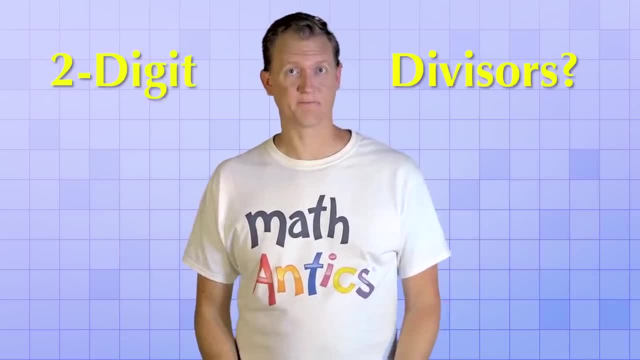 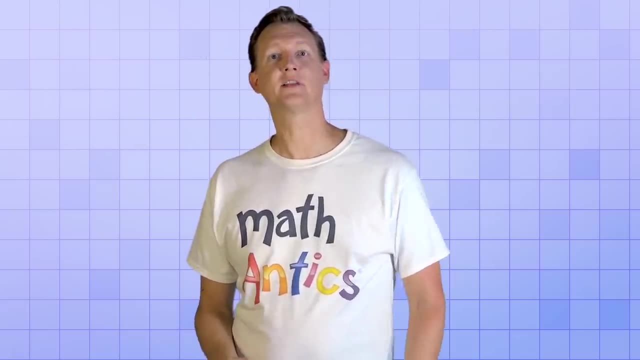 Okay, but how does that relate to 2 digit divisors? Ah, as you'll see, 2 digit divisors force us to take bigger steps. To see what I mean, let's try solving two new division problems that have the same dividend as before, but two new divisors. 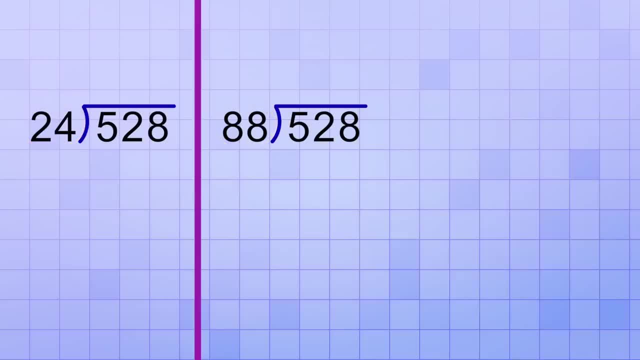 and both of these are two-digit divisors. In this first problem, we could start by asking how many 24s will fit into 5.. But since our divisor now has two digits, we already know that no one-digit chunk of the dividend will be big enough for that to divide into. 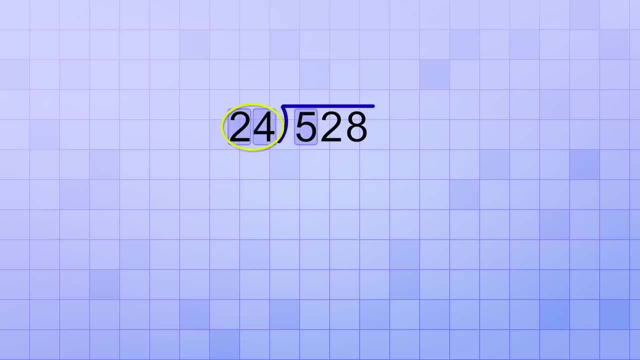 So because we have a two-digit divisor, we automatically need to group the first two digits and ask how many 24s will make 52.. This is trickier because multiples of 24 are not on our multiplication table. Instead, we have to figure it out by estimating or good guessing. 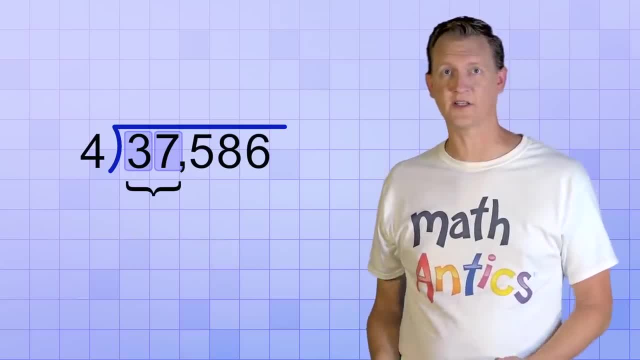 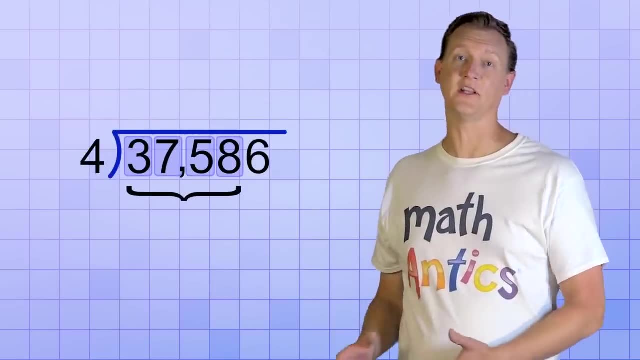 It's much easier because all of the answers to those smaller division steps can be found on the multiplication table, which you have memorized right. But when we have to go 3 or 4 digits at a time, it's a lot harder to figure out the answer of each step. 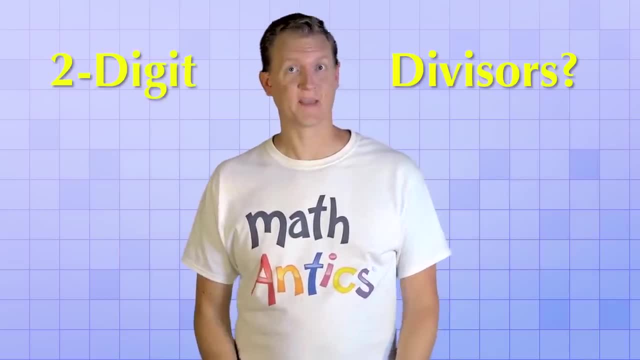 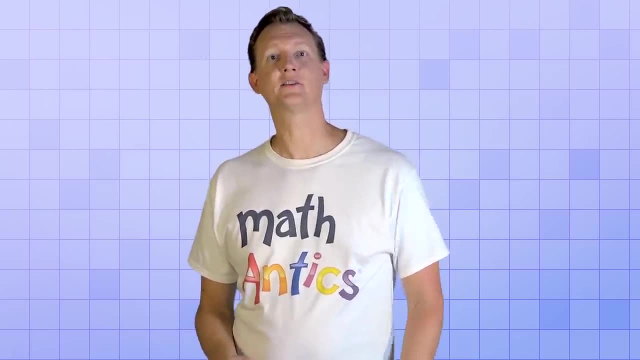 Okay, but how does that relate to two-digit divisors? Ah, as you'll see, two-digit divisors force us to take bigger steps. To see what I mean, let's try solving two new division problems that have the same dividend as before, but two new divisors. 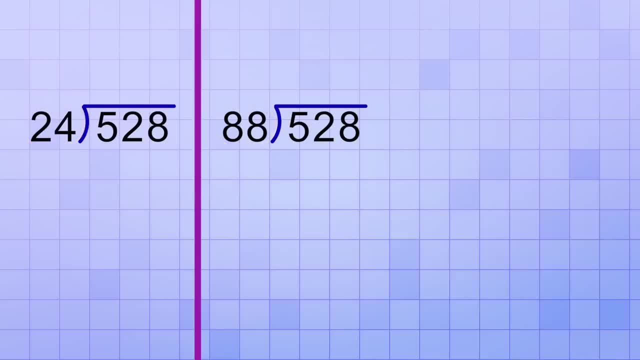 and both of these are two-digit divisors. In this first problem, we could start by asking how many 24s will fit into 5.. But since our divisor now has two digits, we already know that no one-digit chunk of the dividend will be big enough for that to divide into. 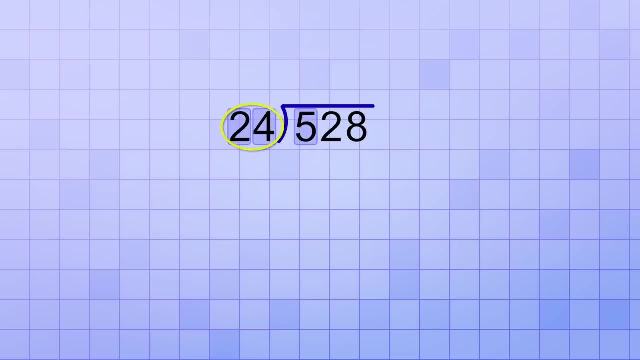 So because we have a two-digit divisor, we automatically need to group the first two digits and ask how many 24s will make 52.. This is trickier because multiples of 24 are not on our multiplication table. Instead, we have to figure it out by estimating or a good guessing. 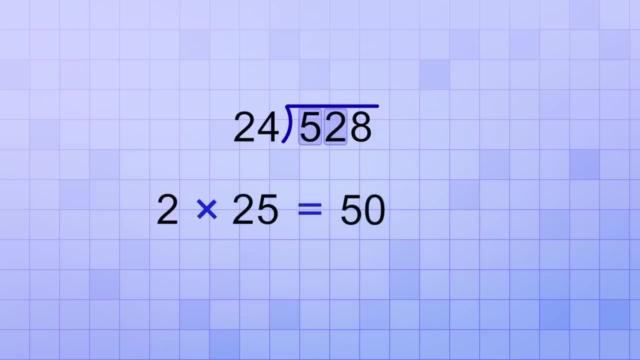 Because we know that 2 times 25 would be 50,. 2 is a really good estimate for the first digit of our answer. 2 times 24 is 48, and then when we subtract 48 from 52,, we get a remainder of 4.. 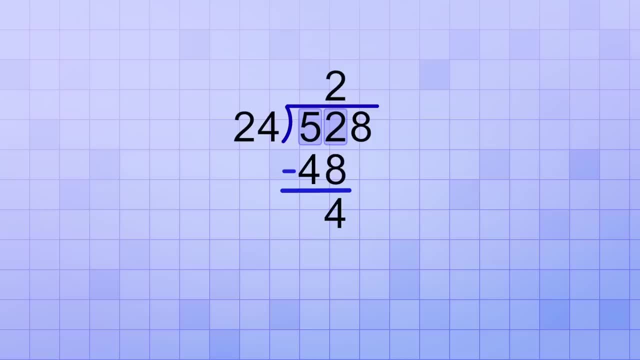 OK, so far, so good. We've already dealt with the first two digits of the dividend, So now we bring down the last digit to join the remainder and ask how many 24s will make 48.. That's easy, It's 2 again. 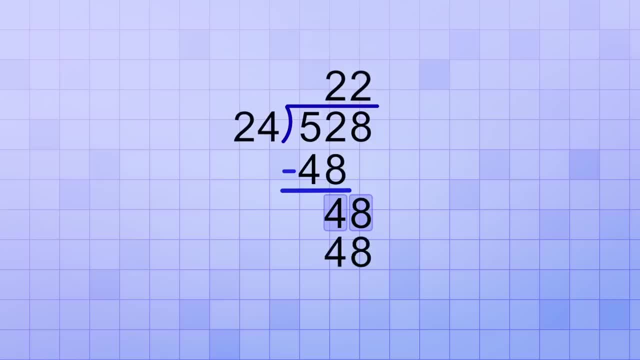 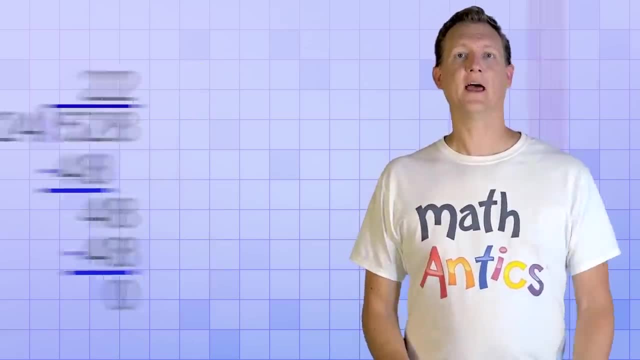 Because we just saw that 2 times 24 is 48. So that will leave no remainder. So the answer to this first two-digit divisor problem is 22.. Now let's have a look at the next problem. It's also got a two-digit divisor and a two-digit divisor. 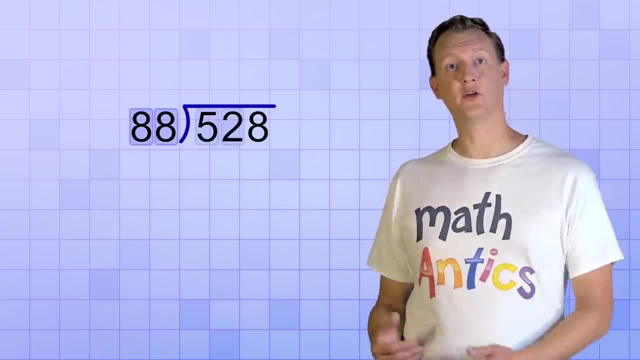 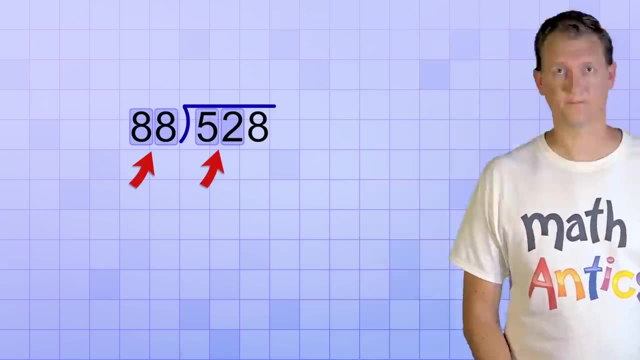 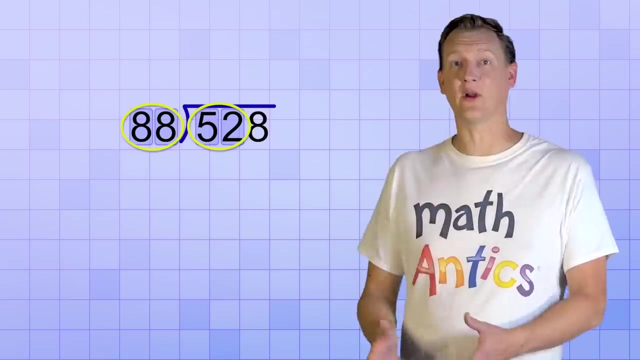 So we'll start the same way. We'll start with a two-digit chunk of our dividend and ask: how many 88s will it take to make 52 or almost 52?? Uh oh, See the problem: Even though both are two digits, this won't work, because 88 is already greater than 52.. 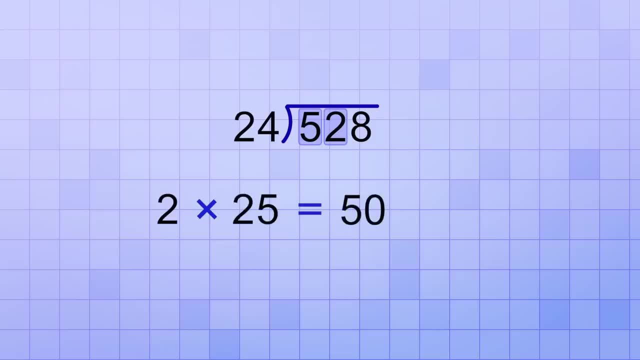 Because we know that 2 times 25 would be 50,. 2 is a really good estimate for the first digit of our answer. 2 times 24 is 48, and then when we subtract 48 from 52,, we get a remainder of 4.. 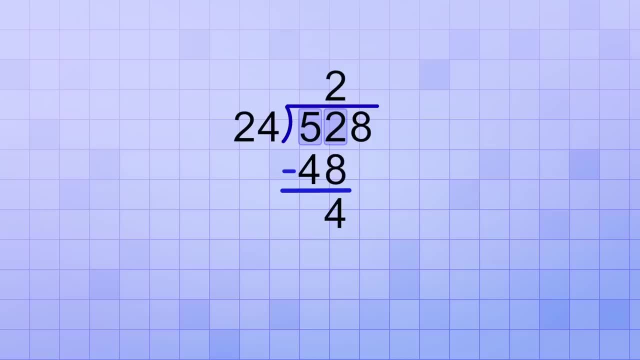 OK, so far, so good. We've already dealt with the first two digits of the dividend, so now we bring down the last digit to join the remainder and ask how many 24s will make 48.. That's easy, it's 2 again. 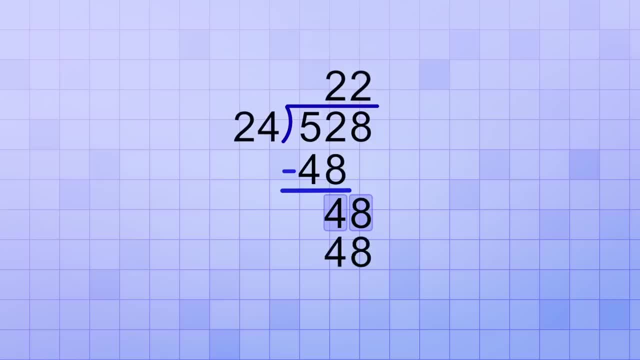 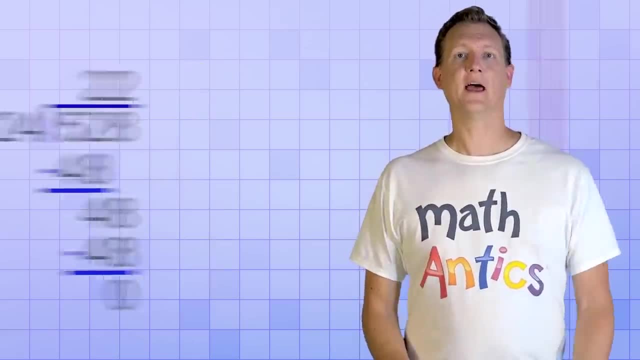 Because we just saw that 2 times 24 is 48, so that will leave no remainder. So the answer to this first two-digit divisor problem is 22.. Now let's have a look at the next problem. It's also got a two-digit divisor, but it's not a divisor. 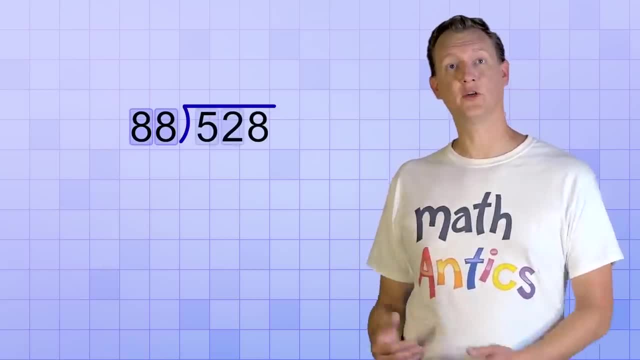 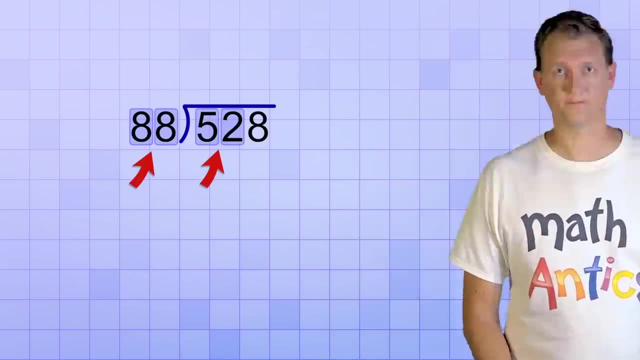 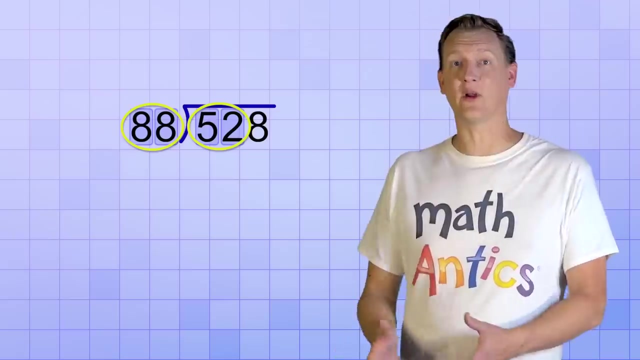 So we'll start the same way. We'll start with a two-digit chunk of our dividend and ask: how many 88s will it take to make 52 or almost 52?? Uh oh, See the problem: Even though both are two digits, this won't work, because 88 is already greater than 52.. 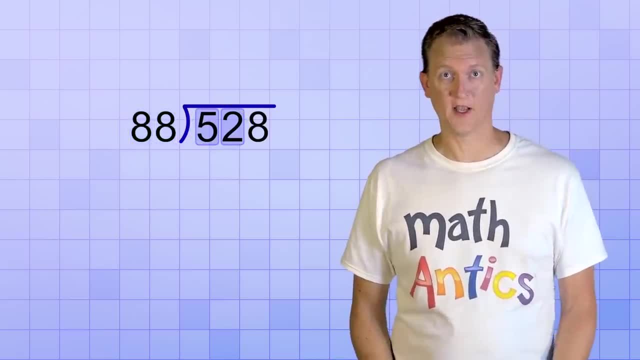 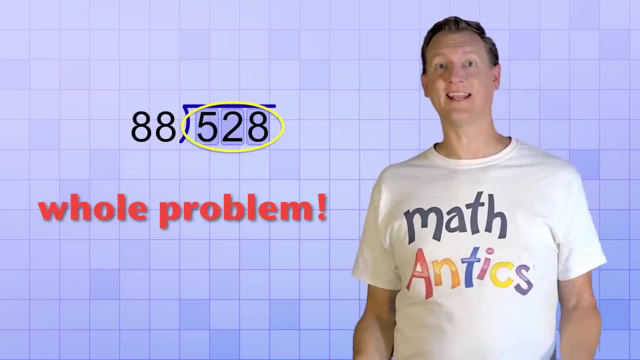 And that means we're going to have to take an even bigger chunk of this dividend. We need to group the first three digits together, But that's just like doing the whole problem at once without breaking it into any steps. Yup, and that's why division problems with big divisors can get difficult. 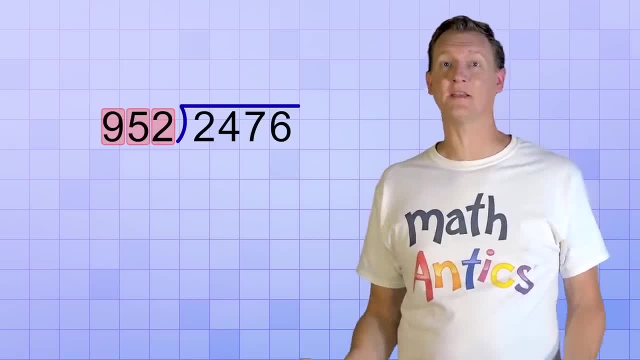 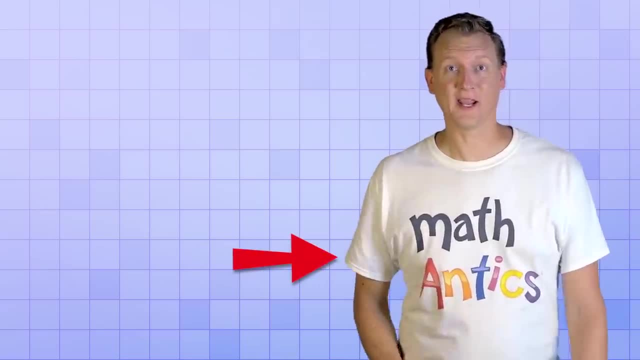 When you have a two or three-digit divisor, each step might be as big as the whole long division problem and it can take a lot of trial and error to figure it out. In fact, if we had our way here at Math Antics, 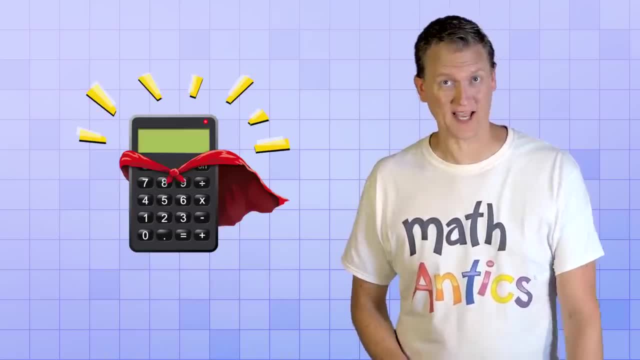 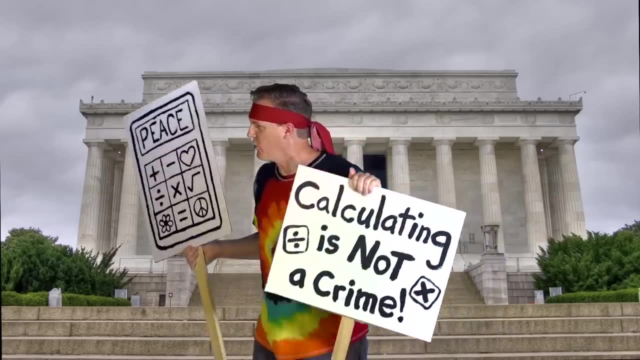 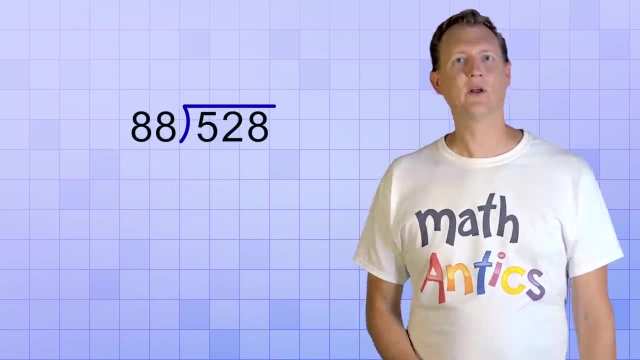 when division problems get that complicated, we'd just let students use calculators to solve them. What do we want Calculators? When do we want them? Whenever we have long division with two or more digit divisors, Okay. but what if we don't get our way and you need to solve this problem without a calculator? 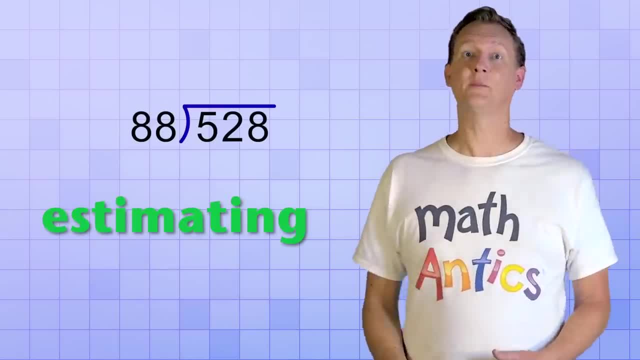 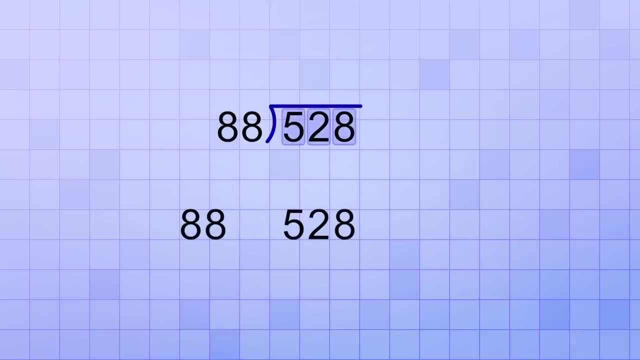 What's the best strategy? Well, a little estimating will help us make much better guesses at our answer. The numbers 88 and 528 are kind of hard to work with, but if we made estimates of those numbers, like if we changed them to 90 and 500,? 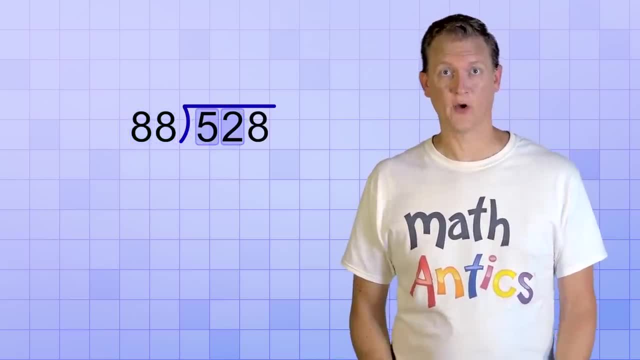 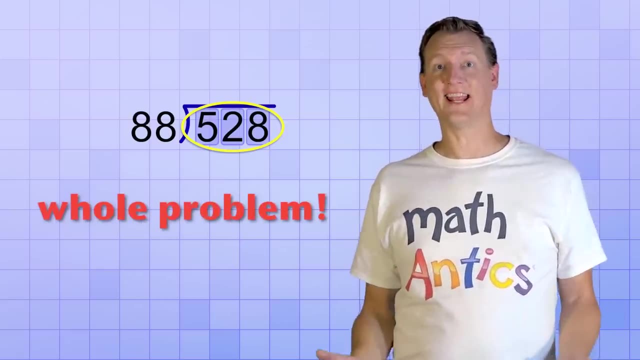 And that means we're going to have to take an even bigger chunk of this dividend. We need to group the first three digits together, But that's just like doing the whole problem at once without breaking it into any more Any steps. Yup, and that's why division problems with big divisors can get difficult. 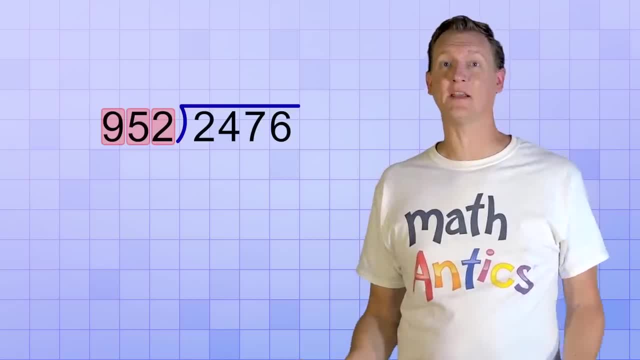 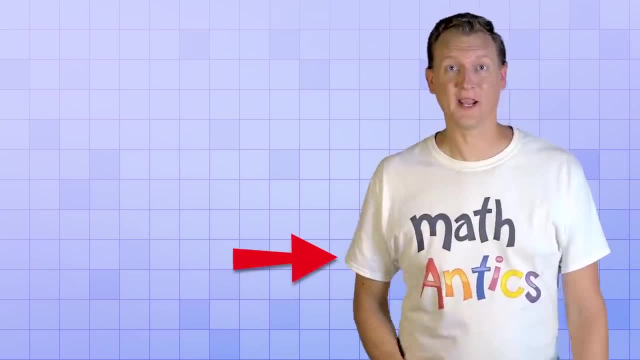 When you have a two or three digit divisor, each step might be as big as the whole long division problem and it can take a lot of trial and error to figure it out. In fact, if we had our way here at Math Antics, 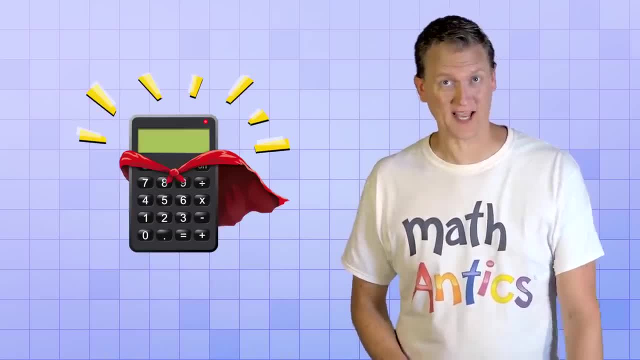 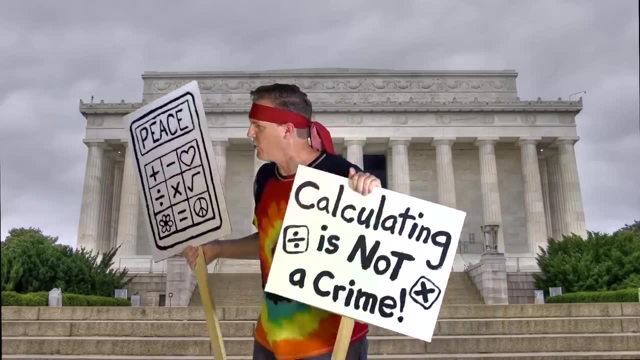 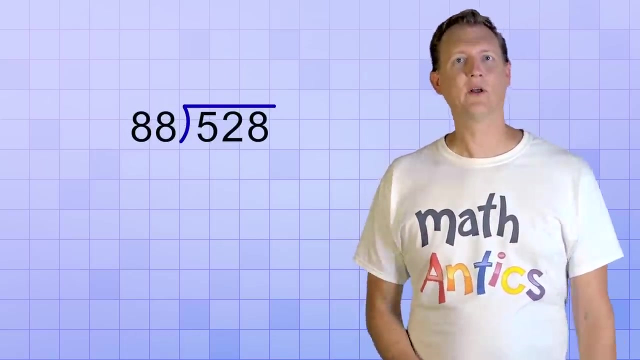 when division problems get that complicated, we'd just let students use calculators to solve them. What do we want Calculators? When do we want them? Whenever we have long division with two or more digit divisors, Ok. but what if we don't get our way and you need to solve this problem without a calculator? 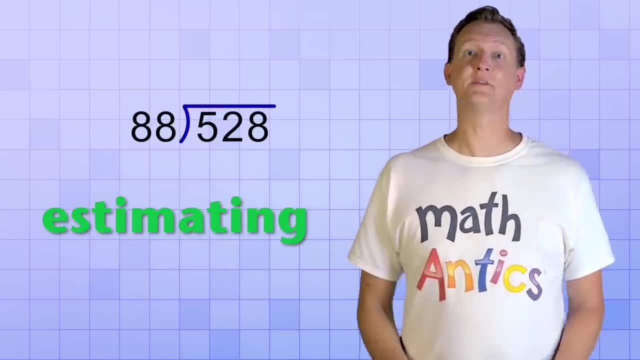 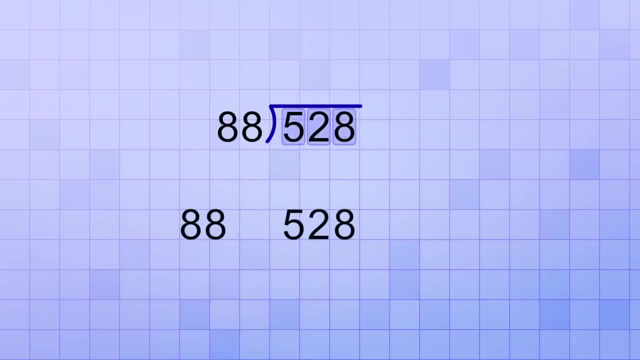 What's the best strategy? Well, a little estimating will help us make much better guesses at our answer. The numbers 88 and 528 are kind of hard to work with, But if we made estimates of those numbers, like if we changed them to 90 and 500,? 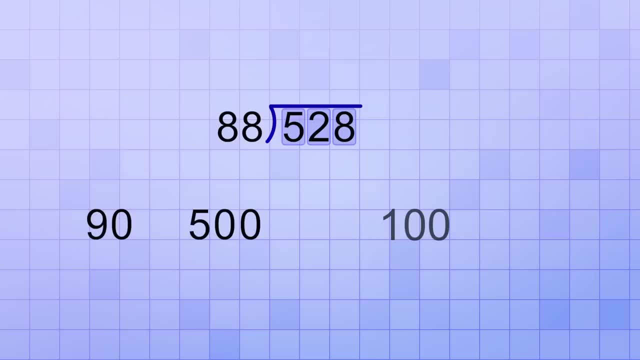 that would make it easier to estimate the answer. Since 100 would divide into 500 exactly 5 times, that means that 90 will divide into 500 exactly 5 times. That means that 90 will divide into 500 at least that many times. 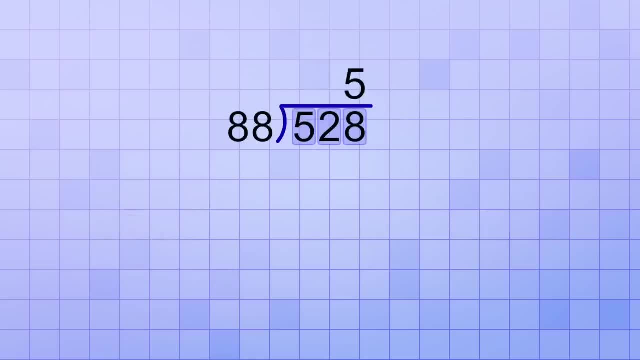 So let's make 5 our first estimate for the answer. To check to see how good that estimate is, we multiply 5 by 88 and then subtract that from 528 to see what the remainder is. Now, 5 times 88 is kind of tricky on its own. 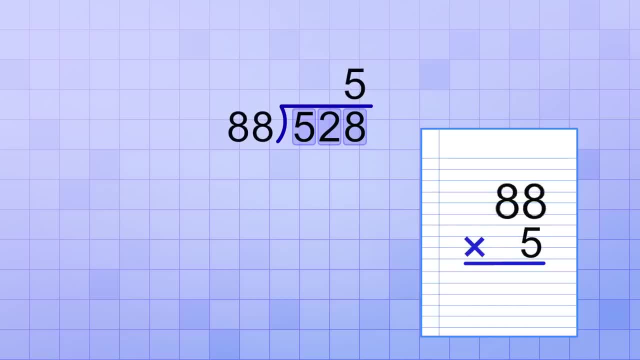 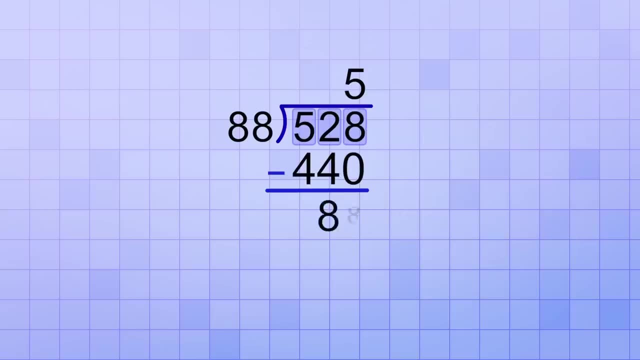 so you may want to use scratch paper to work it out: 5 times 88 is 440, and when we subtract 440 from 528, we get a remainder of 88.. Hmm, looks like our estimate was too low. Whenever the remainder is greater than or equal to the divisor, 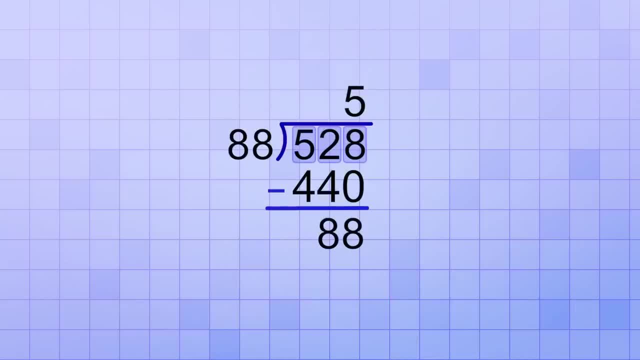 it means we underestimated the answer. In fact, since our remainder is equal to the divisor, it means we could have divided exactly one more 88 into 528.. So we should have picked 6.. And if you multiply 6 times 88, you'll see that it's 528. 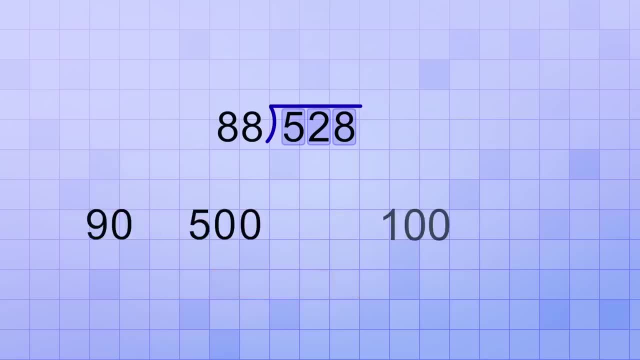 that would make it easier to estimate the answer. Since 100 would divide into 500 exactly five times, that means that 90 would divide into 500 exactly five times. that means that 90 would divide into 500 exactly five times and 90 will divide into 500 at least that many times. 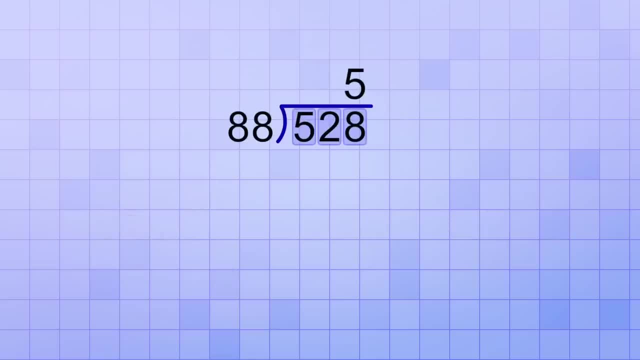 So let's make 5 our first estimate for the answer. To check to see how good that estimate is, we multiply 5 by 88 and then subtract that from 528 to see what the remainder is. Now, 5 times 88 is kind of tricky on its own. 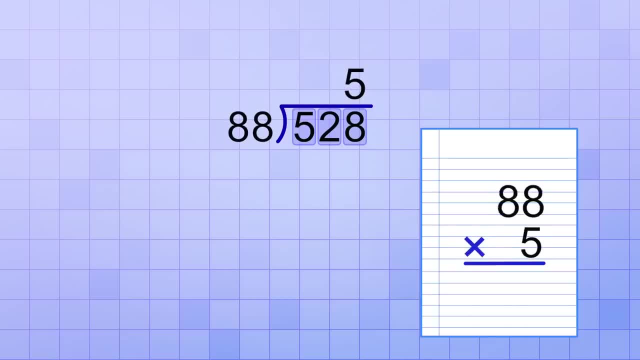 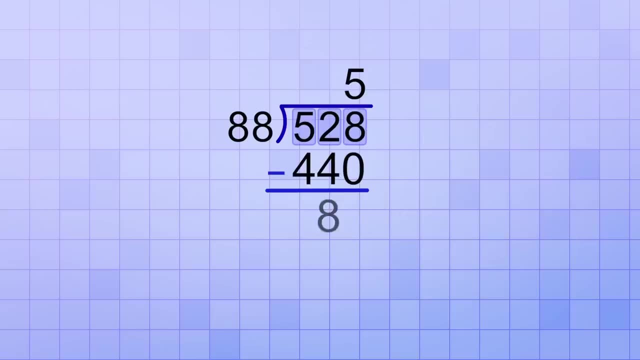 so you may want to use scratch paper to work it out: 5 times 88 is 440, and when we subtract 440 from 528, a remainder of 88. Hmm… looks like our estimate was too low. Whenever the remainder is greater than or equal to the divisor, it means we underestimated the answer. 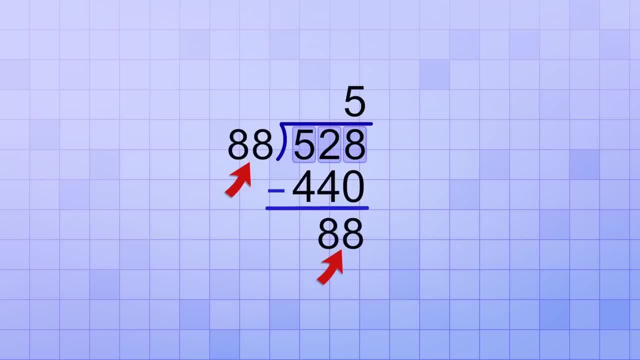 In fact, since our remainder is equal to the divisor, it means we could have divided exactly one more 88 into 528.. So we should have picked 6.. And if you multiply 6 times 88, you'll see that it's 528.. 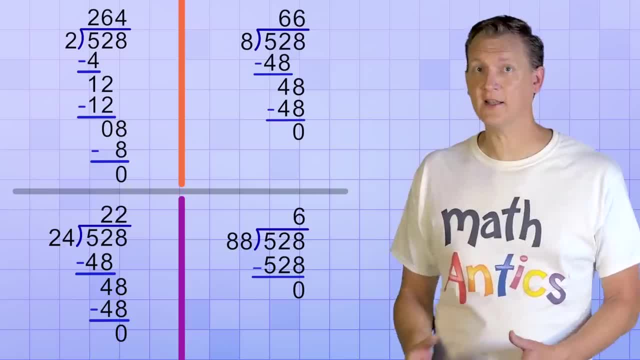 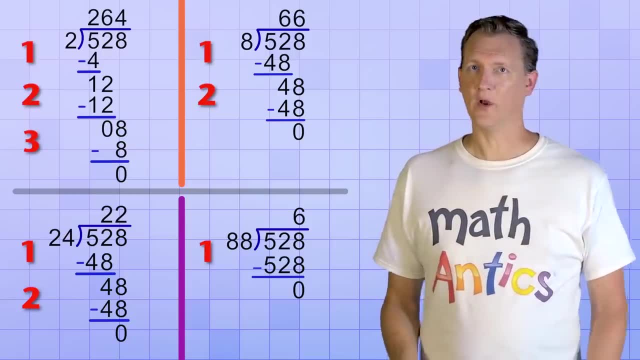 So, as you can see, even though the division procedure is basically the same, in all these cases, the value of the divisor makes a big difference on our division steps, Whenever the divisor is bigger than the part of the dividend that we're trying to divide. 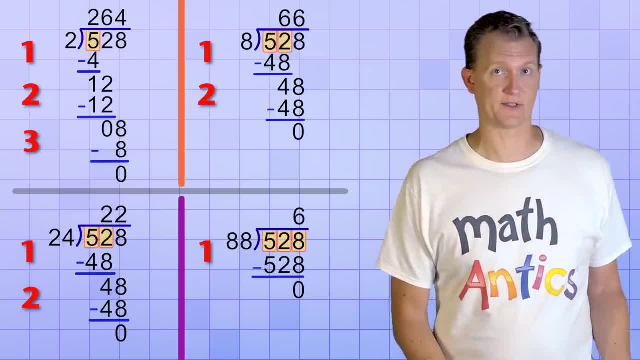 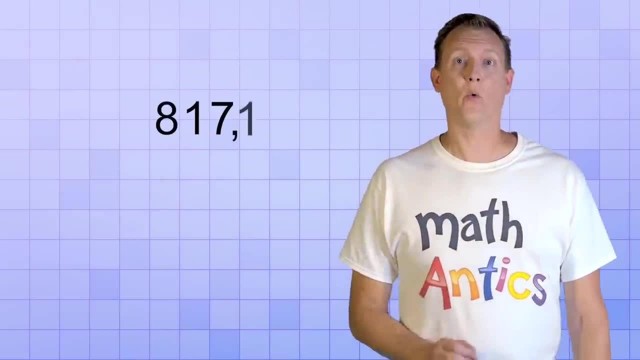 it means that we need to group more digits and take bigger division steps. Let's try one more, much longer two-digit divisor problem: 800, 17,000, 152 divided by 38.. I'm going to work through this kind of problem. 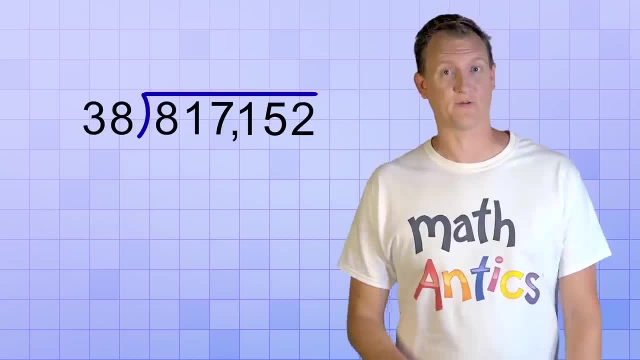 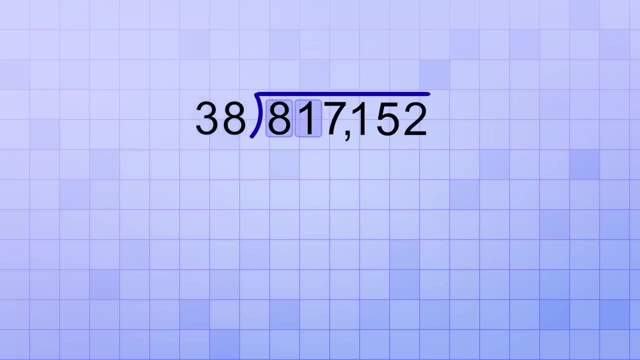 It's kind of fast so you may want to re-watch it a couple times if you have trouble following it. Since we have a two-digit divisor, we start with the first two digits of the dividend and ask: how many 38's will it take to make 81?? 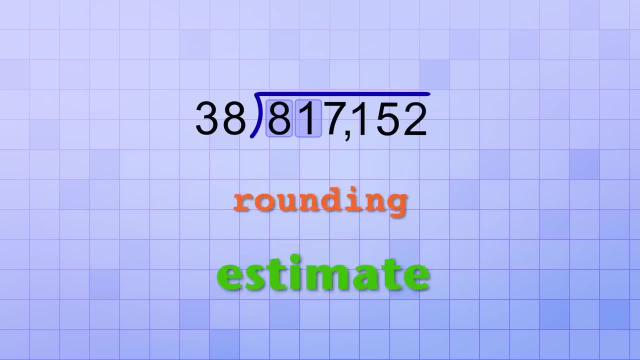 Again, we're going to use rounding to help us estimate the answer: 38 is close to 40 and 81 is really close to 80., And since 80 is 2 times 40, my estimate for the first answer digit will be 2.. 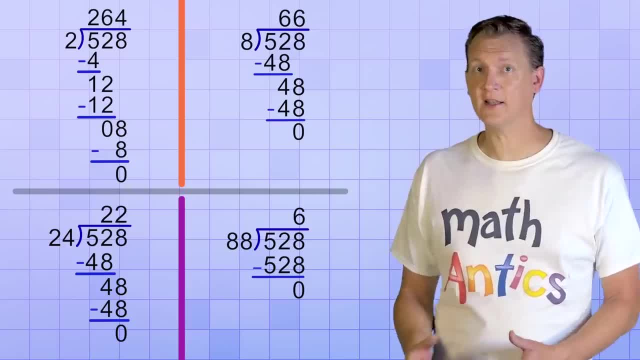 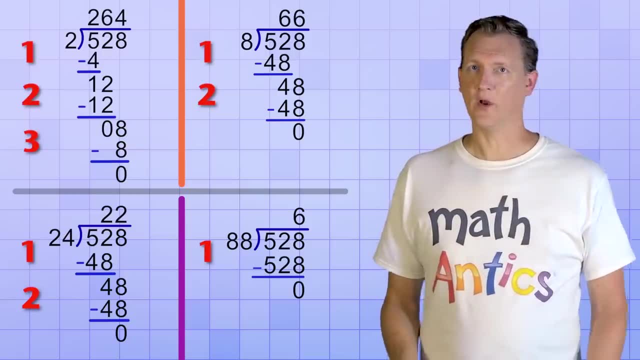 So, as you can see, even though the division procedure is basically the same, in all these cases, the value of the divisor makes a big difference on our division steps, Whenever the divisor is bigger than the part of the dividend that we're trying to divide. 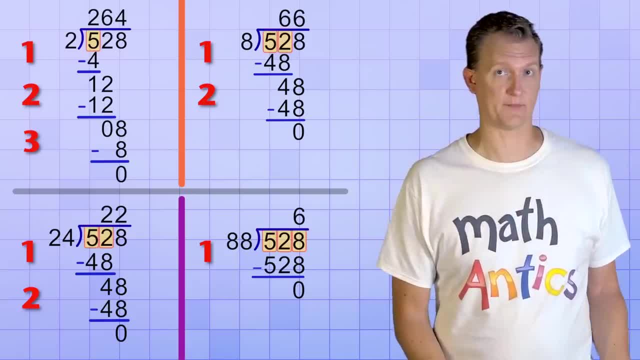 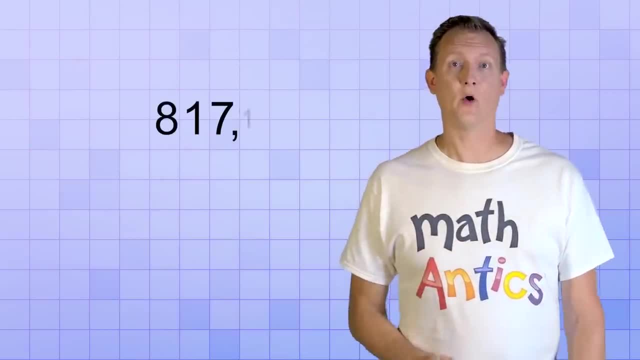 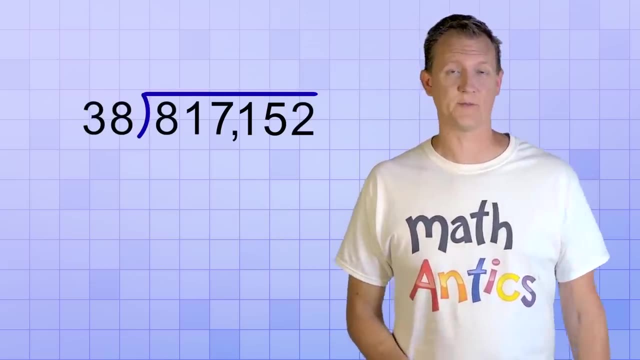 it means that we need to group more digits and take bigger division steps. Let's try one more, much longer 2-digit divisor problem: 817,152 divided by 38.. I'm going to work through this kind of fast so you may want to rewatch it a couple times. 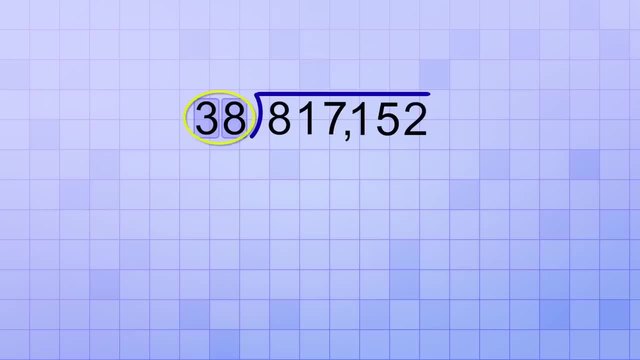 if you have trouble following it. Since we have a 2-digit divisor, we start with the first 2 digits of the dividend and ask: how many 38s will it take to make 81?? Again, we're going to use rounding to help us estimate the answer. 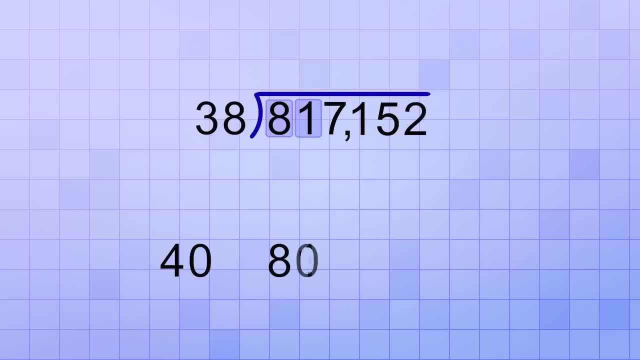 38 is close to 40 and 81 is really close to 80. And since 80 is 2 times 40, my estimate for the first answer digit will be 2.. 2 times 38 equals 76. And 81 minus 76 equals 1.. 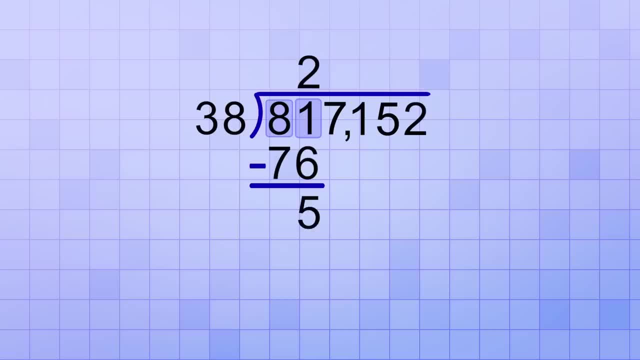 Minus 76 leaves a remainder of 5.. We know our estimate was just right, because 5 is less than our divisor of 38. Now we move on to the next digit. We bring a copy of it down and combine it with our 5 and ask: 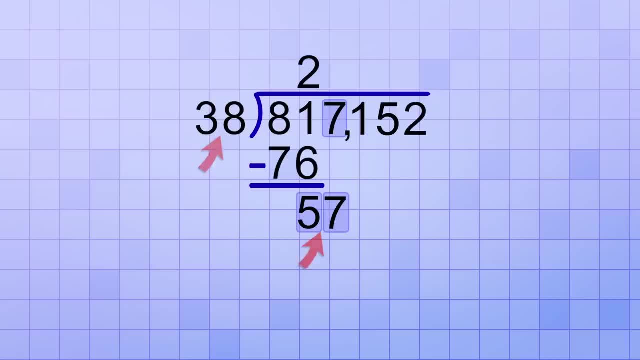 how many 38s will it take to make 57? That one's easier to estimate just 1,, because it's easy to see that 2 38s would be too big. 1 times 38 equals 38. And 57 minus 38 leaves a remainder of 19.. 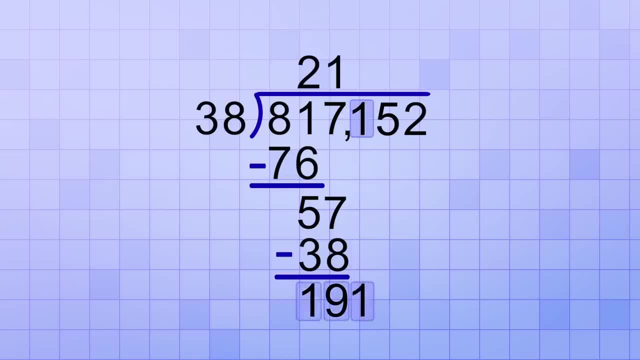 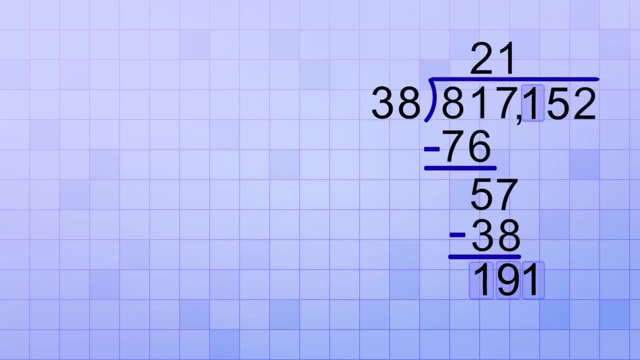 On to the next digit. We bring down a copy of the 1 and now we ask: how many 38s will it take to make 191?? That's a bit tougher To estimate. I'll round those numbers to 40 and 200. 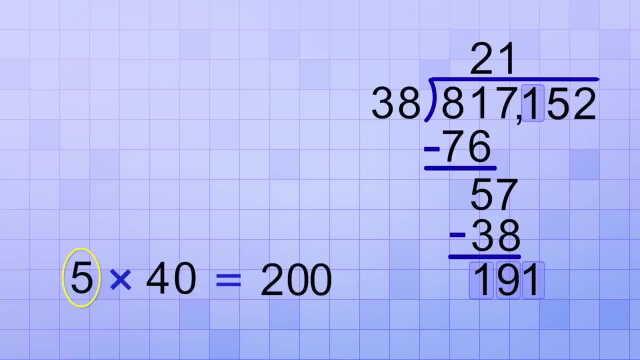 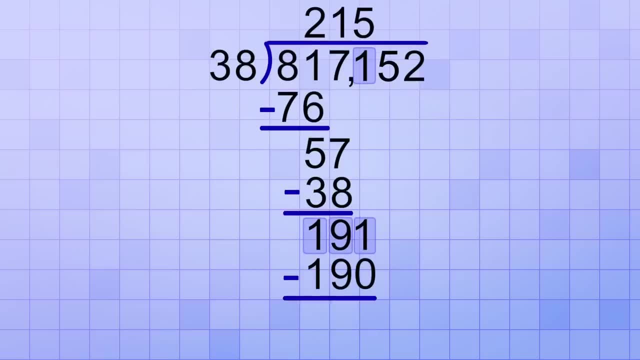 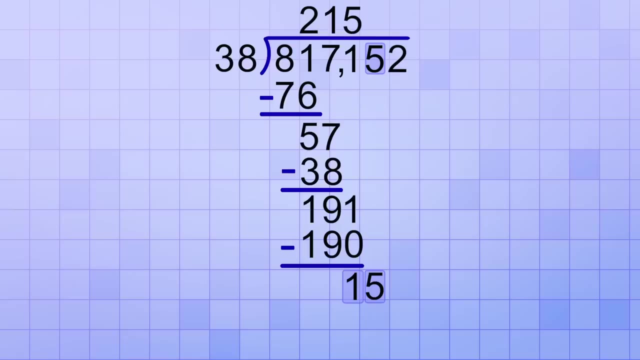 And I know that 5 40s makes 200, so 5 is my estimate. for the next answer, digit 5 times 38 equals 190. And 191 minus 190 leaves a remainder of 1.. Moving on, We move on to the next digit and ask. 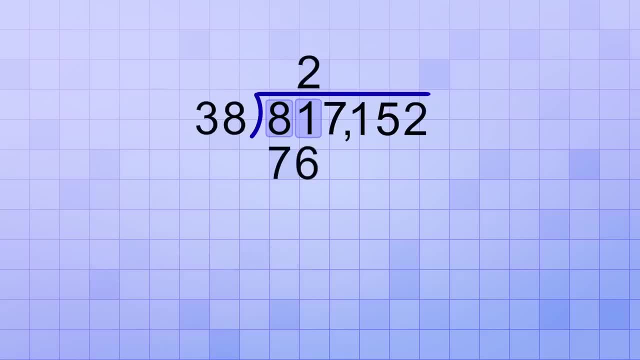 2 times 38. Equals 76. And 81 minus 76 leaves a remainder of 5.. We know our estimate was just right, because 5 is less than our divisor of 38. Now we move on to the next digit. 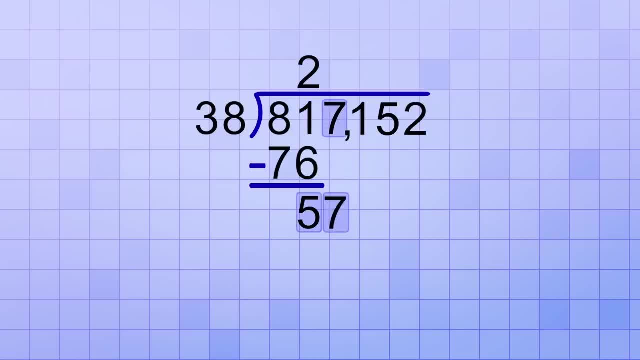 We bring a copy of it down and combine it with our 5 and ask: how many 38's will it take to make 57?? That one's easier to estimate. just 1, because it's easy to see that 2 38's would be too big. 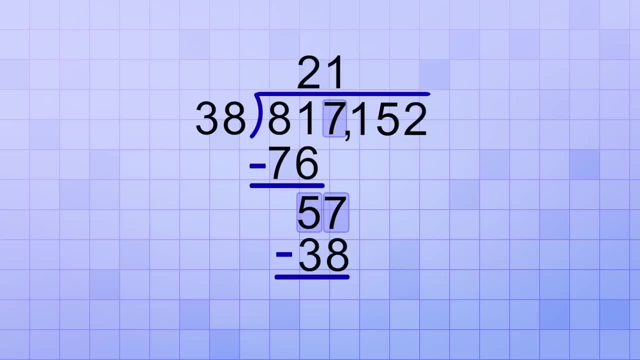 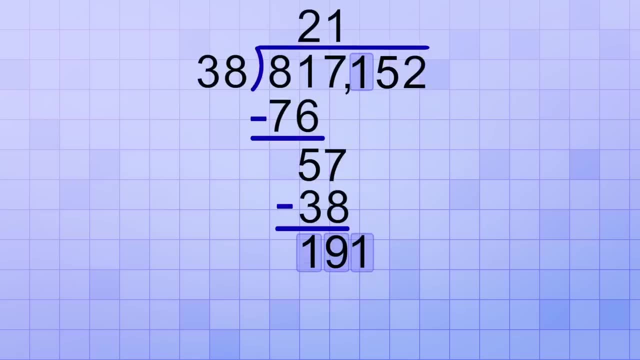 1 times 38 equals 38. And 57 equals 1.. Minus 38 leaves a remainder of 19.. On to the next digit. We bring down a copy of the 1, and now we ask: how many 38's will it take to make 191?? 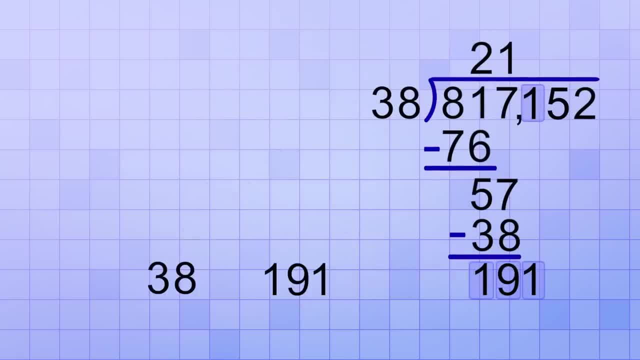 That's a bit tougher To estimate. I'll round those numbers to 40 and 200.. And I know that 5, 40's makes 200, so 5 is my estimate. for the next answer: digit 5 times 38 equals 190.. 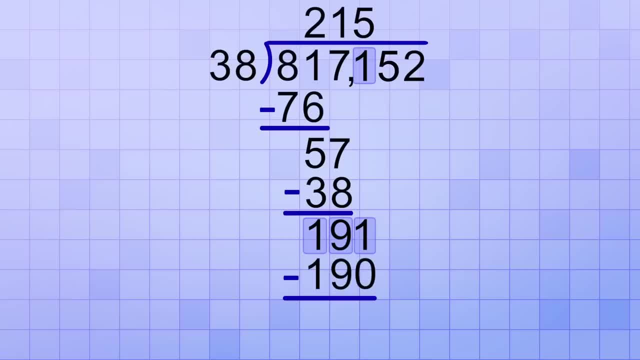 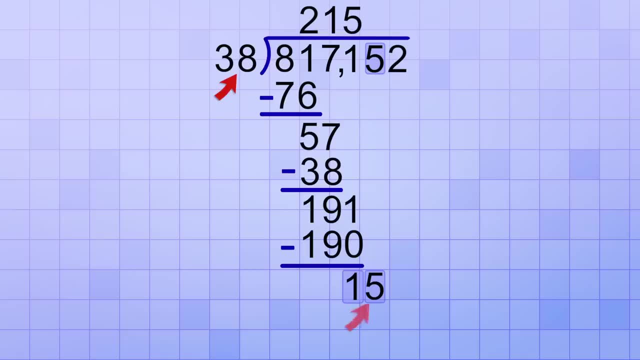 And 191 minus 190 leaves a remainder of 1.. Moving on, We bring down a copy of our next digit and ask: how many 38's will it take to make 15?? Uh oh, 15 isn't big enough to be divided by 38.. 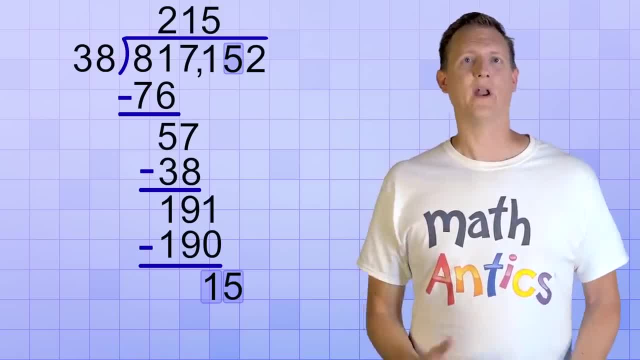 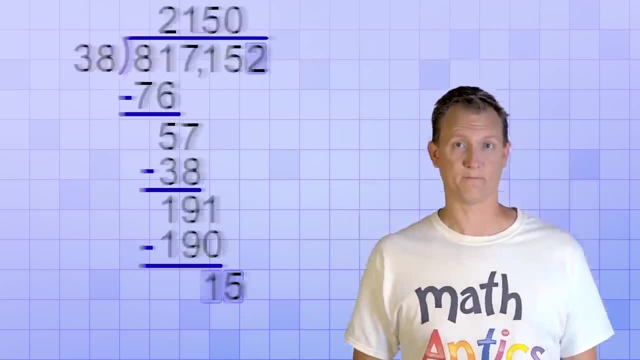 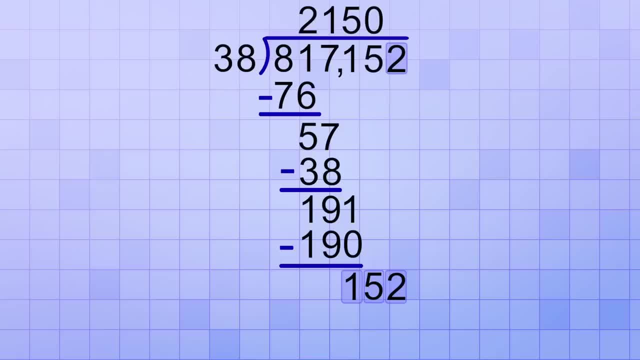 Now we ask how many 38's will it take to make 152?? Now we ask how many 38's will it take to make 152?? To estimate this one, I'm going to round those numbers to 40 and 160. 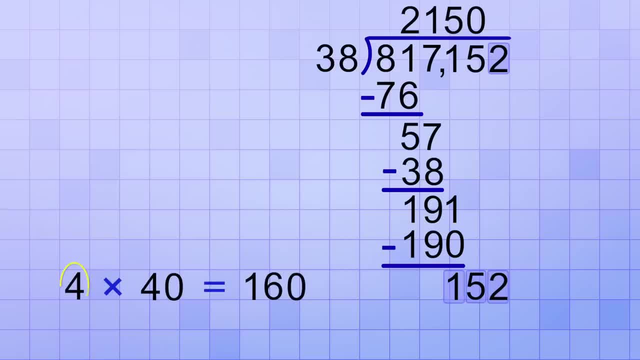 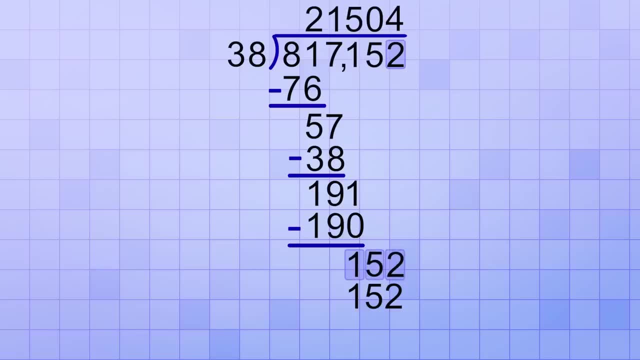 And since 4 times 40 equals 160, I'll put 4 in the answer line as my estimate. 4 times 38 equals 152. And 152 minus 152 leaves no remainder And we're done. Wow, that was a lot of work. 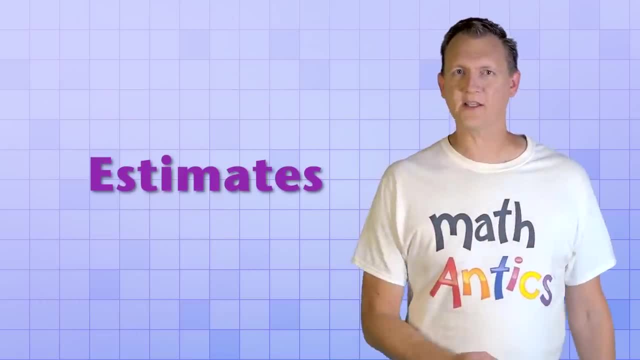 But did you see how much rounding helped us out? We made good estimates each time by rounding the numbers we were working on. We made good estimates each time by rounding the numbers we were working on. We made good estimates each time by rounding the numbers we were working on. 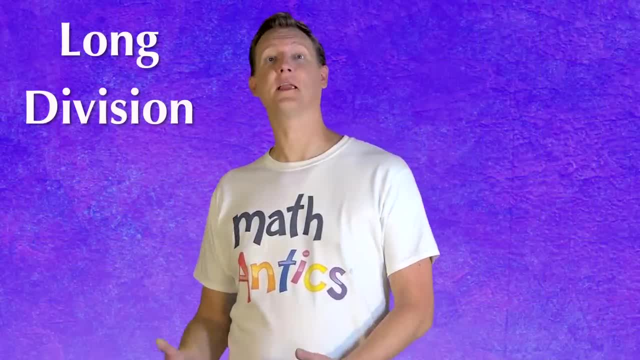 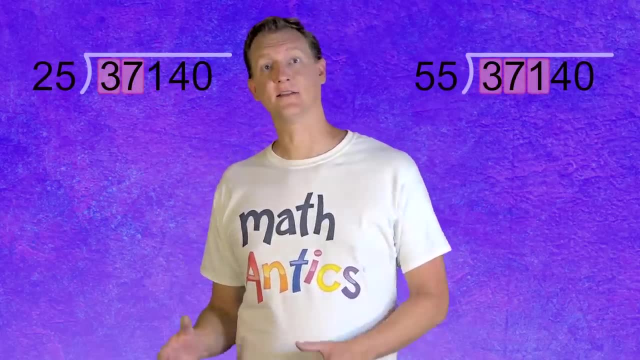 Alright, now you know that the long division procedure works the same for two-digit divisors. It's just that each division step will involve two or three digits of the dividend, And since each of those bigger steps is harder to figure out, you'll want to use estimating to help you find the answers. 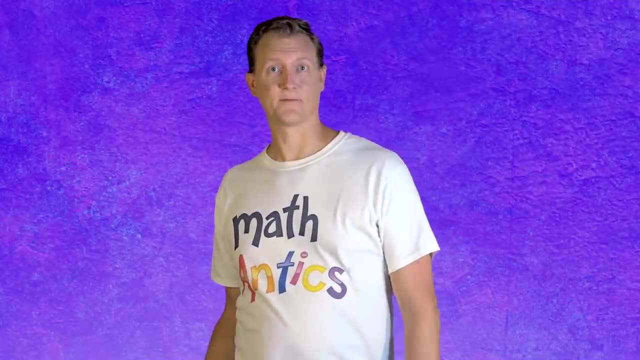 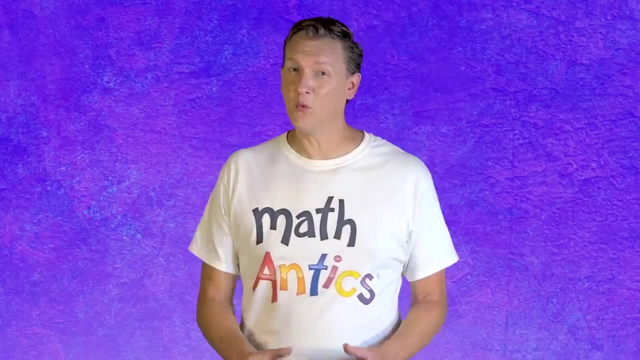 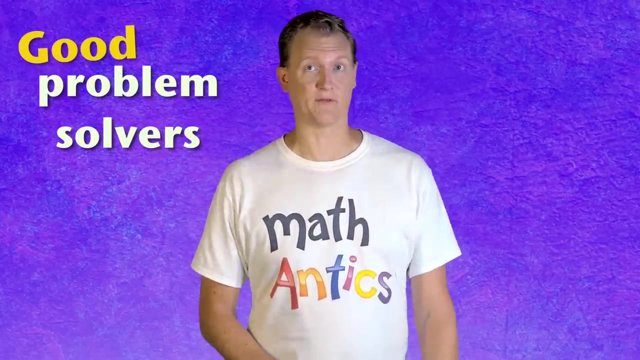 And while it's good to know how to do complex division problems like this, we still think that complex division problems are a job for your calculator. So try a few practice problems, but don't wear yourself out doing really long division like this. After all, the reason we study math is to become good problem solvers. 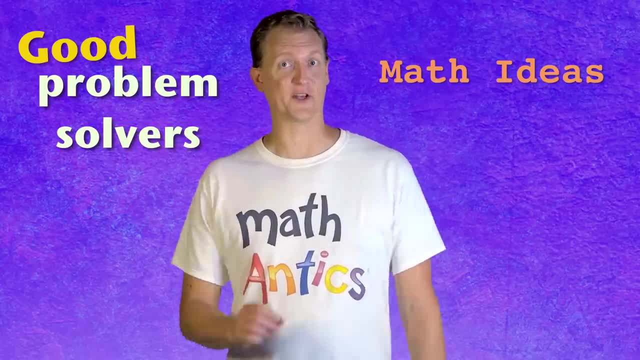 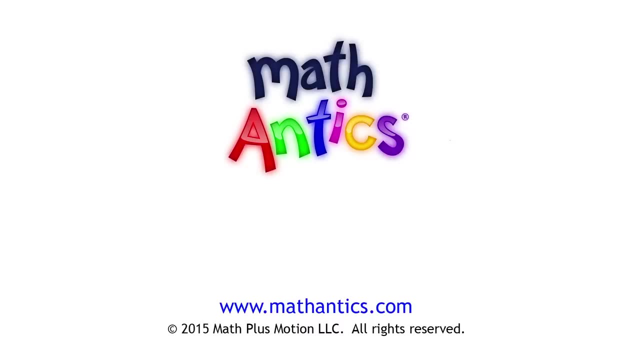 and to be able to understand all sorts of important math ideas, And there's a lot more to math than division. As always, thanks for watching Math Antics and I'll see you next time. Learn more at wwwmathanticscom. 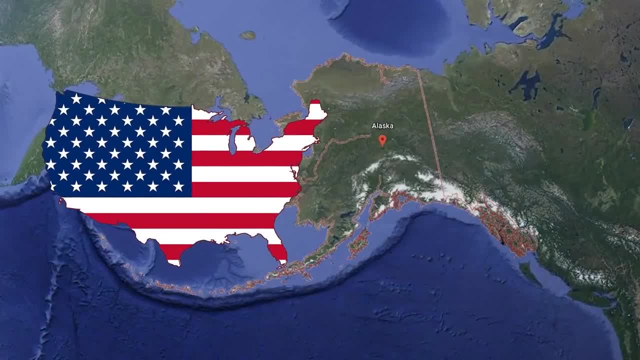 Have you ever wondered why Alaska is a part of the United States despite bordering Canada? Well, in 1741, Russia discovered Alaska and proceeded to colonize it for its sea otters, and it was also seen as cool to have a colony at that time. But fast forward to the 1850s and Russia now wanted 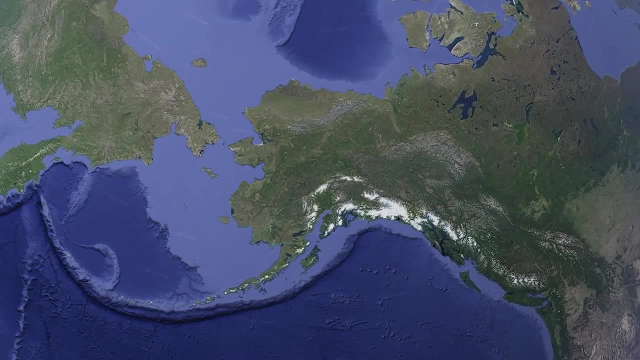 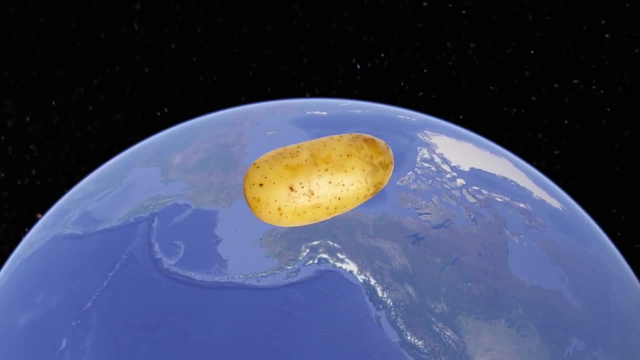 to sell Alaska. So that begs the question: why? One reason for this is that the sea otters had been overhunted, making Alaska unprofitable. It was also too far north for the settlers to grow food there, making it unlikely for Alaska to have a large population. It was also hard to manage due 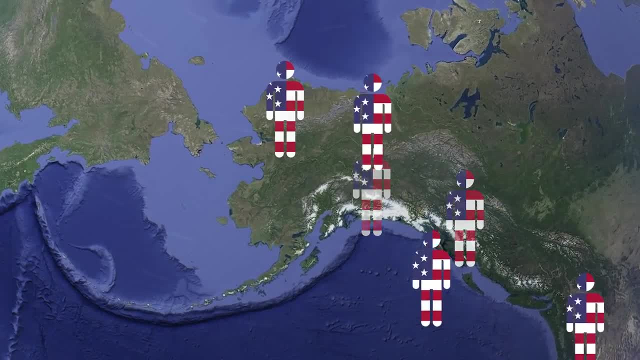 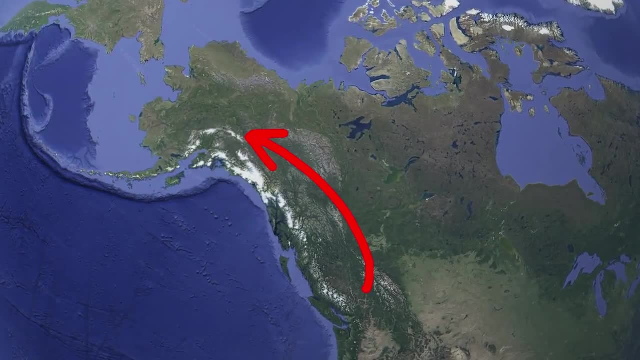 to its distance and Russia worried that an influx of Americans searching for gold was inevitable. Plus, Russia was afraid of Britain taking advantage of Alaska's vulnerability by taking it over through British Columbia. I mean, Alaska only had 800 settlers at its peak. so Britain taking it over would have been easy. But the main reason why Russia wanted to sell Alaska was due to the Crimean War, which Russia had lost and gotten into a lot of debt for. The question now is why sell to the United States and not say Canada? Well, Russia didn't want to sell Alaska. 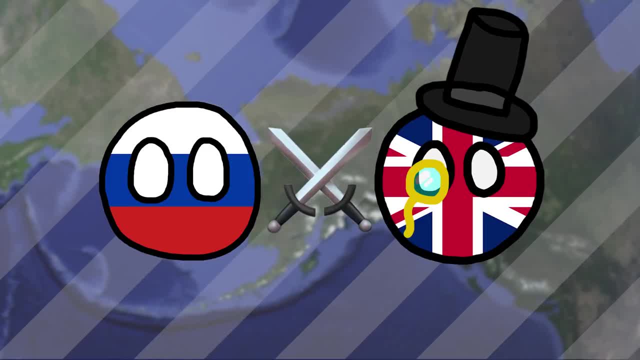 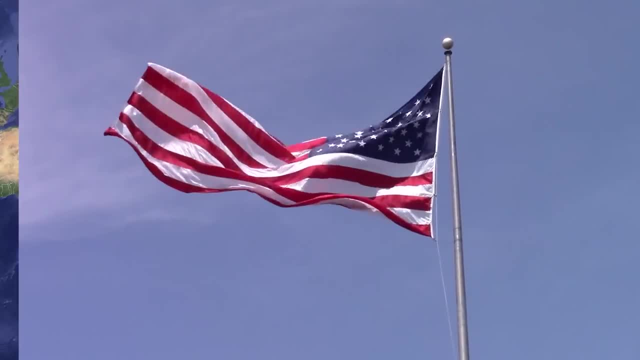 had been able to sell Alaska to the United States, and Russia and Britain were rivals. Plus, they just fought each other during the Crimean War, so that wasn't going to be an option. Instead, they offered Alaska to the United States because it could offset Britain's power in